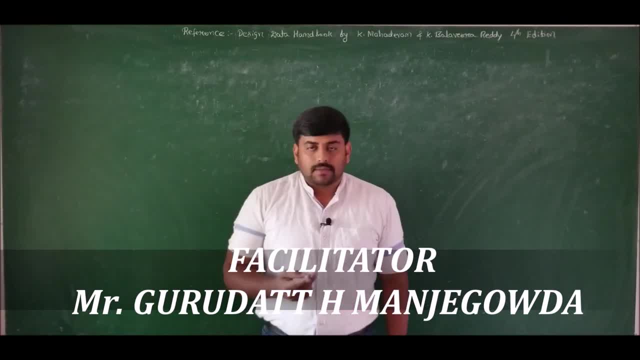 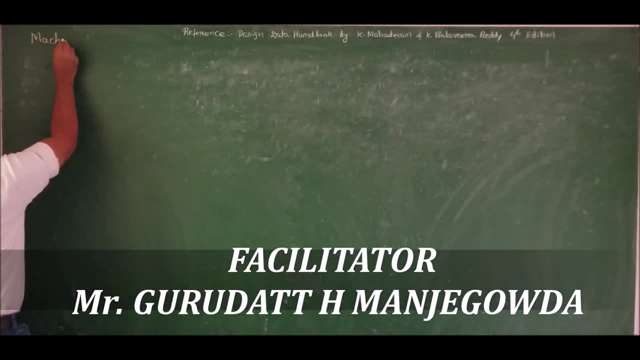 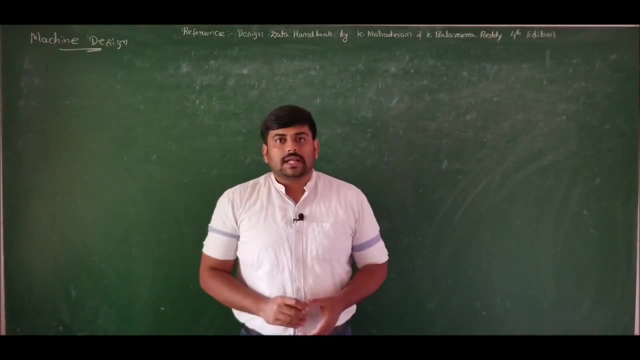 in designing the mechanical members. Come, let us begin the new subject, that is Machine Design, from today's lecture. Machine, Today's lecture. let us understand what is the meaning of machine design. what are the steps involved in design of machine elements? what is that? 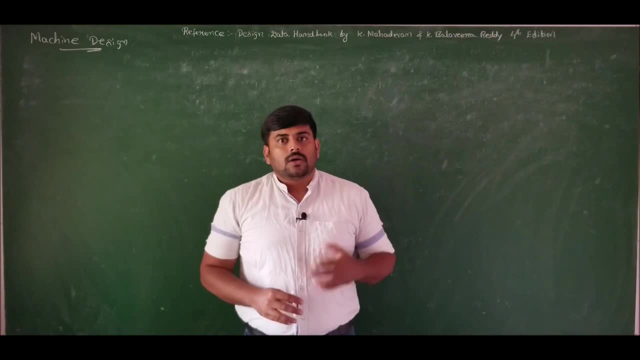 I am going to offer in this course on machine design and what are all the modules, what are the contents in it, and also I will recapture the properties of engineering materials and speak a few words about them, About codes and standards, in today's lecture Coming for this course: Machine Design, Machine. 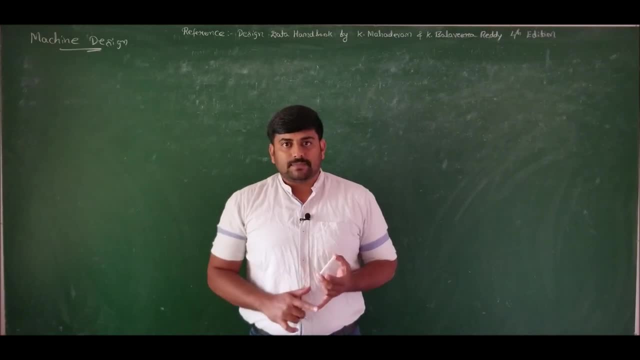 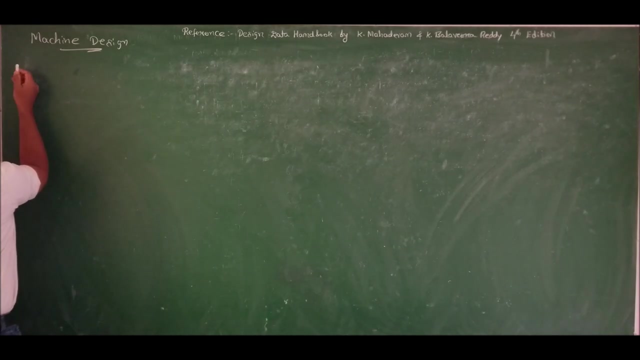 design is defined as application of scientific principles, technical information and imagination in description of machines or mechanical systems to perform the specified operations or functions with high efficiency and economy. If I write down the definition of machine design, it is true that any specific thing it is call as engineering, Machine design is defined. 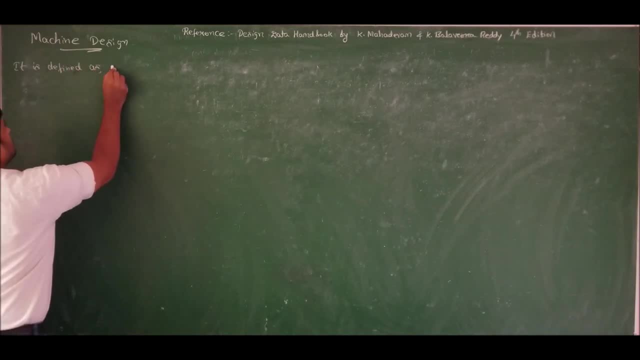 as application of application of first one is scientific principles, Scientific principles. second one is technical information. Second one is technology. Secondly, one is engineering. So what is the technical information, technical information, Especially the technical information. what is the technical knowledge And what is the technical knowledge In the course we are going to talk? 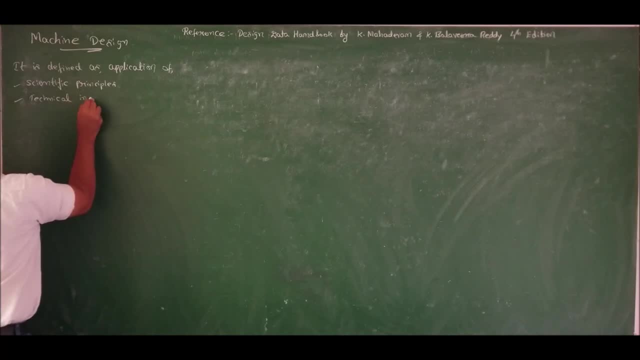 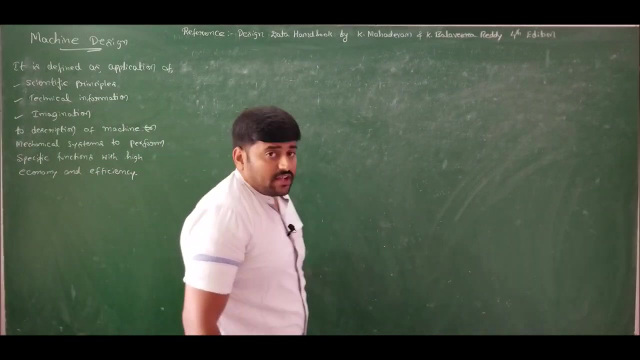 informations. third one is imagination: why we are applying these things. we are applying these things to describe, in description of machine or mechanical systems. machine or mechanical systems to perform specific operations or specific functions with high economy and efficiency, high economy and efficiency. and so machine design is defined as application of scientific principles. 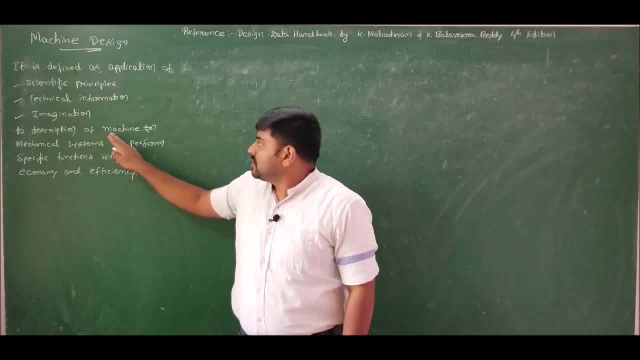 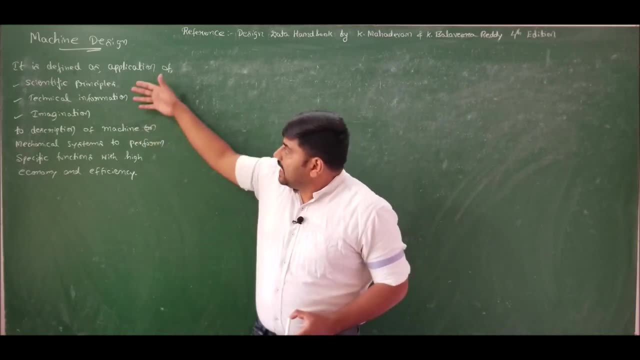 technical principles and scientific principles, and so machine design is defined as application of scientific principles, technical information and imagination in description of machine or mechanical systems to perform specific functions with high economy and efficiency. as the. as the definition itself indicates, we are applying the scientific principles which you have already learnt, for example, N demekиться. 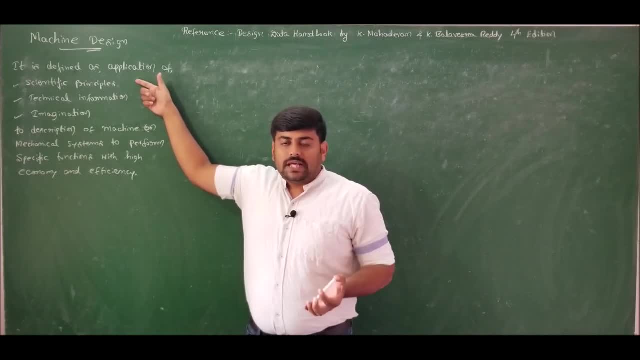 Luta's loss of motion, ‫Bernoulli principle, D A Lambert principle, etc. will apply them in determining the forces acting on various machine members and we will get the technical information. that is, if I want to choose the belt dolphins, there is no belt dolphins and in addition we have additional. 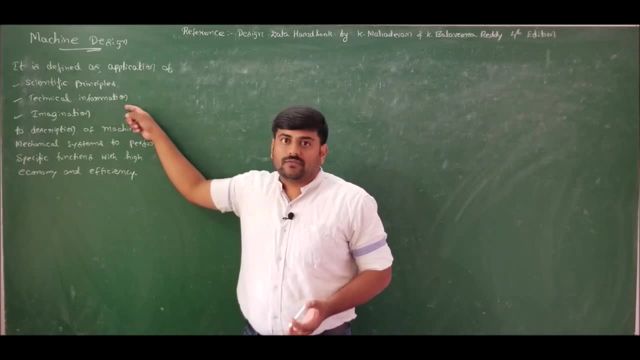 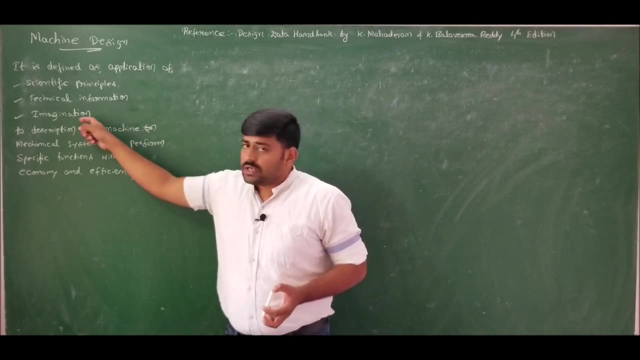 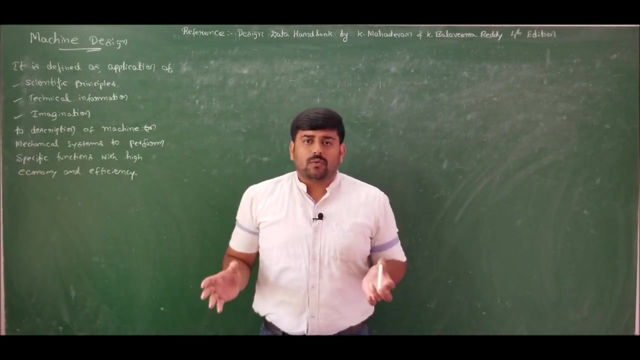 If I want to design a belt drive, I should know the technical information of it, with what material it is made of, what is its tensile strength, what is its ultimate strength. Those things should be known. Coming for imagination, what will be the layout or what will be the dimensions of a belt drive system that I want to fabricate for specified applications? 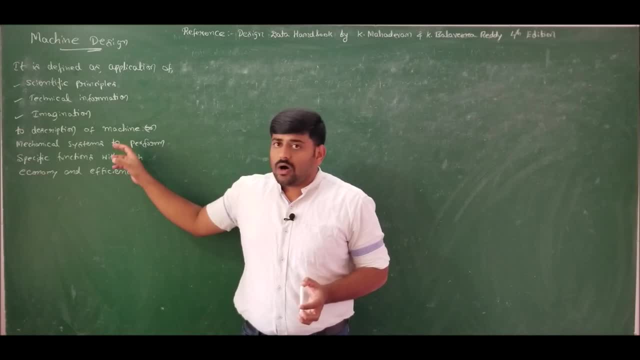 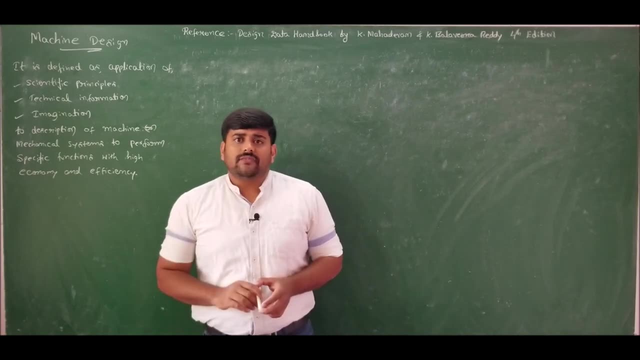 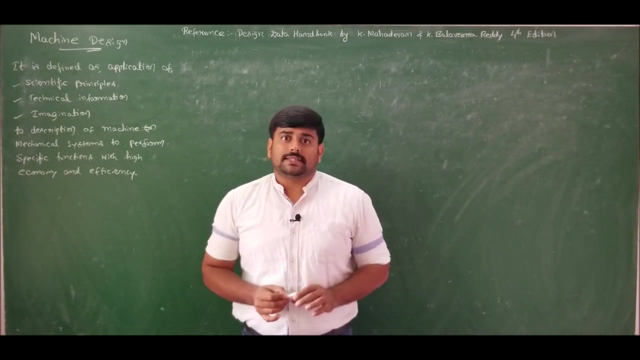 So I am doing these things in order to describe a machine or mechanical system which is intended to perform a specific operation with high economy and efficiency. Now, in this machine design course, we are intended only to design of machine elements, Coming for steps involved in design of machine elements. 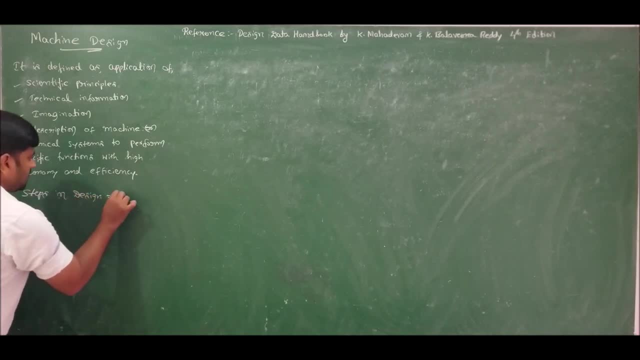 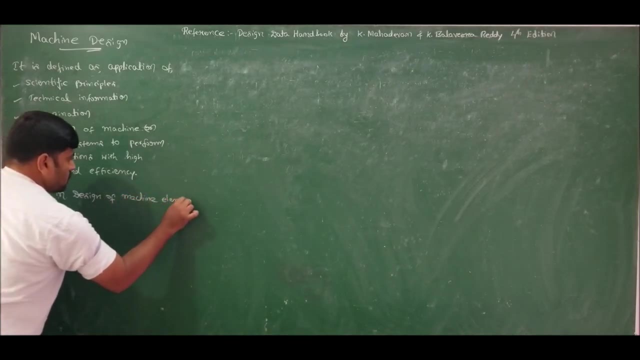 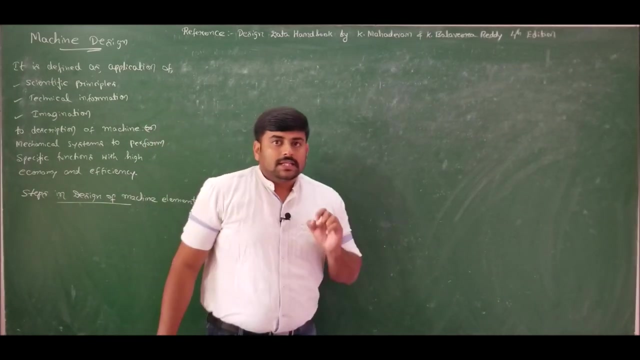 First of all, what is the meaning of machine element? Each part of a machine which has motion relative to another part is termed as machine element, Like if I consider a screw jack. screw jack has cup, tommy, bar, body, etc. 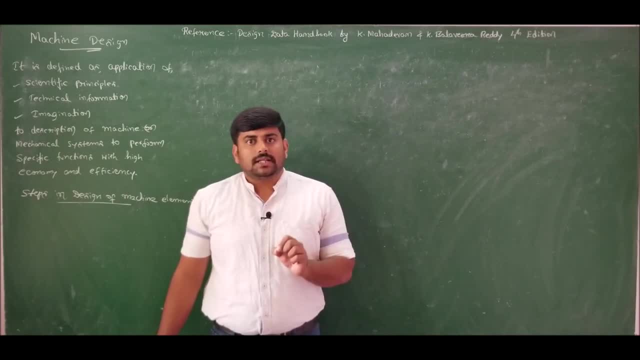 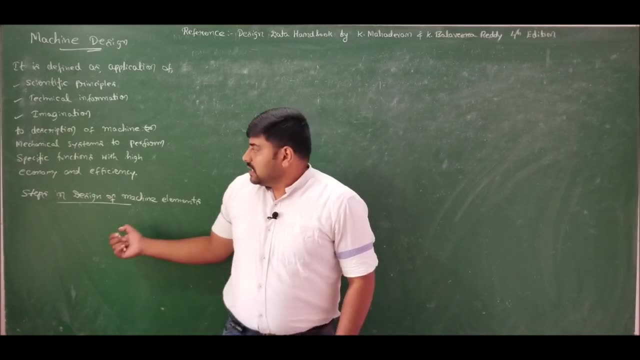 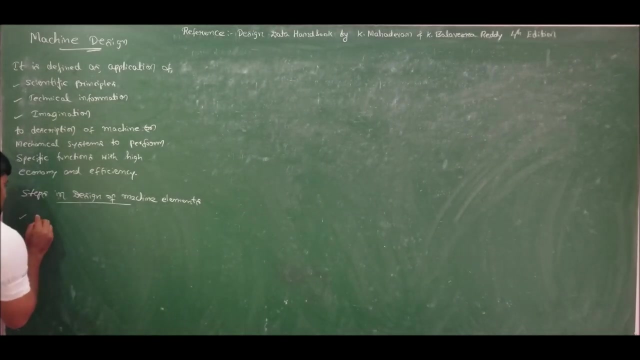 Each of these have motion with respect to another, and these are called as machine elements. So, in designing these things, what are the steps involved is what I am going to discuss now. Coming for steps in design of machine elements, First thing is that we should specify the function of element. 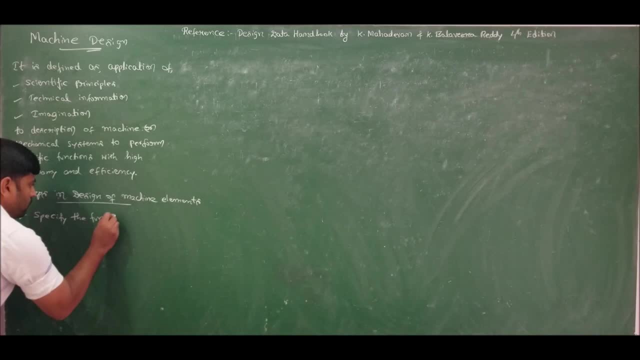 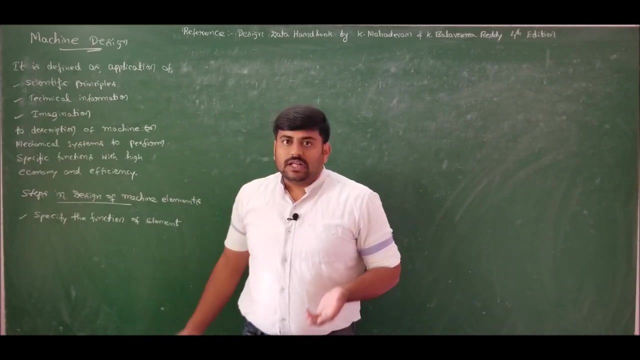 Specify the function of element. Specify the function of element. Whether we are designing the element for power transmission or we are designing the element for lifting a load, etc. Like if I am designing the element for lifting a load like screw jack. 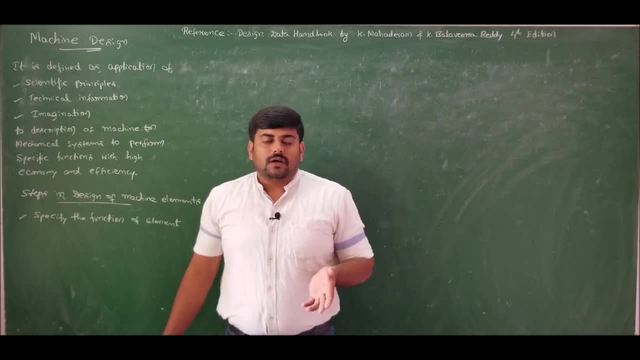 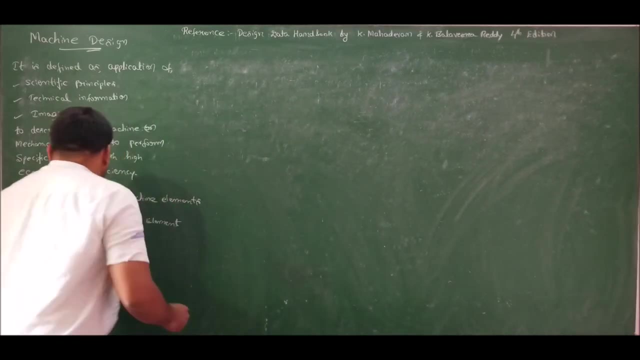 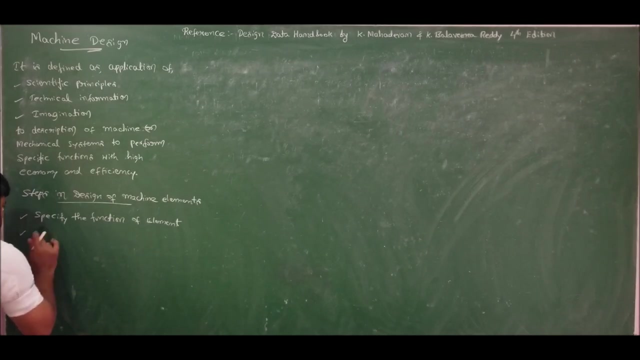 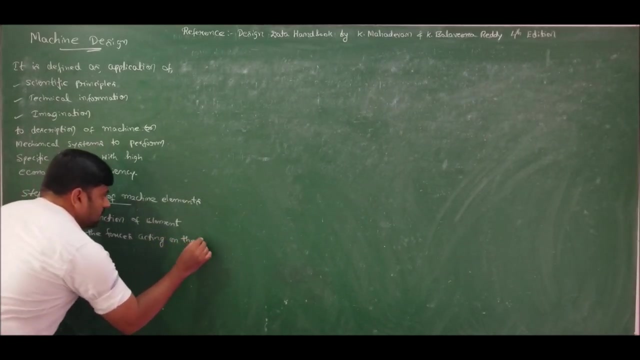 If I am designing an element for power transmission, such as belt drive or gear drive, etc. That I should specify in the first step: Specify the function of element. Second thing is to determine forces acting on the element, That is, determine the forces acting on the element. 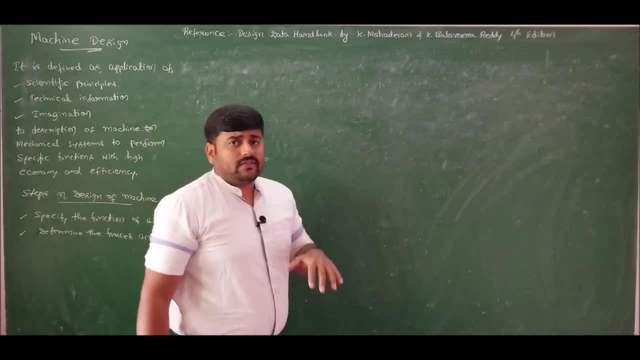 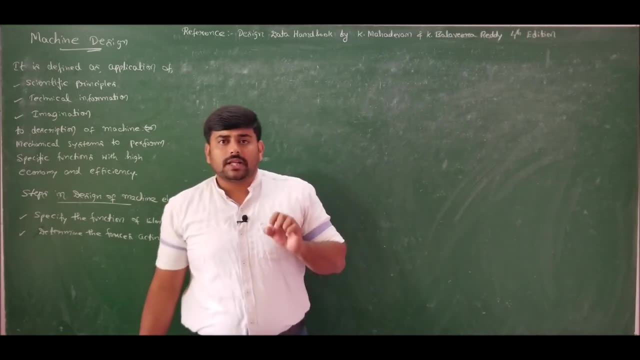 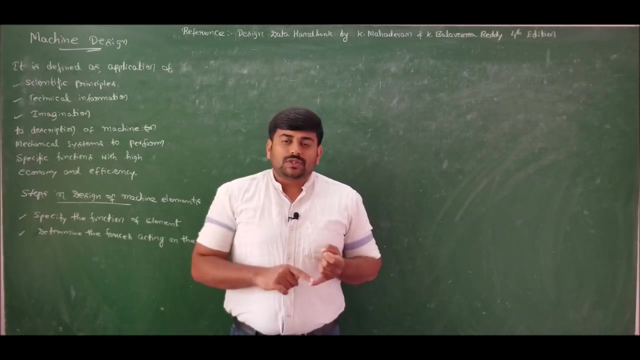 This is very, very important. I should determine what are the various forces acting on the element. This is because of the reason the various forces acting on the element are required to determine what is the stress induced in the element, Coming for various forces- it might be the force due to self weight, dead load or externally applied forces- and what type of forces are acting on it. 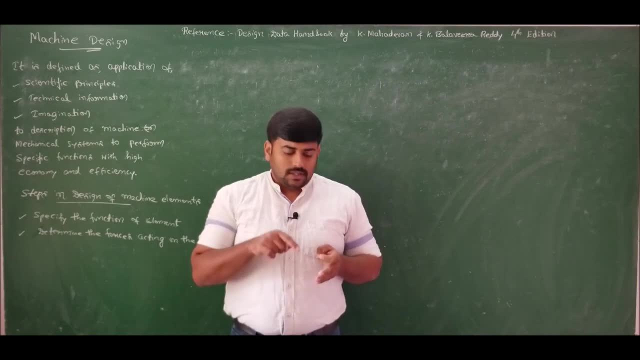 Whether it is gradually applied load, suddenly applied load, or it is subjected for fatigue loading, etc. Example: if I want to design axle, Axle of an automobile are subjected for fatigue loading, Axle of an automobile are subjected for fatigue loading, etc. 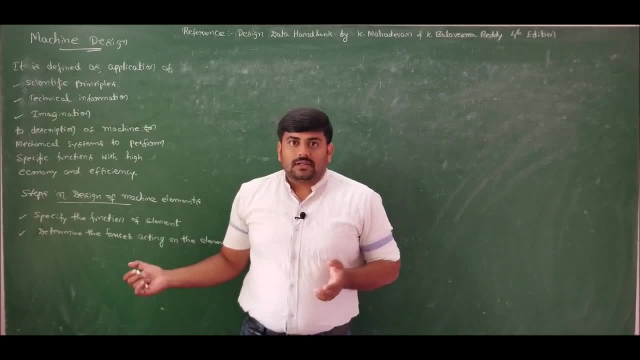 At an Tian-X32asting load. Depending on theceptivity at wel, it should be a fatigue loading as well. Coming for designing of screw jack, It is subjected for concentrated or gradually applied load, That is, it is used to lift an automobile upward in order to change the stiffness, etc. 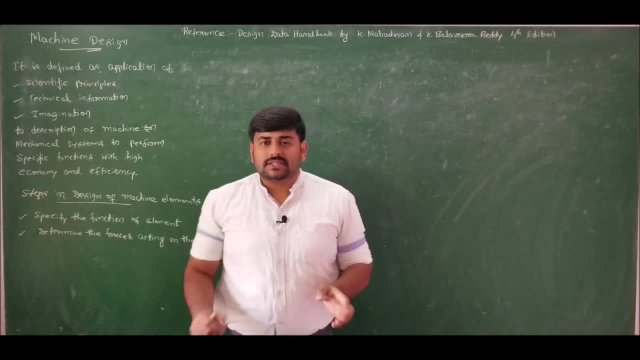 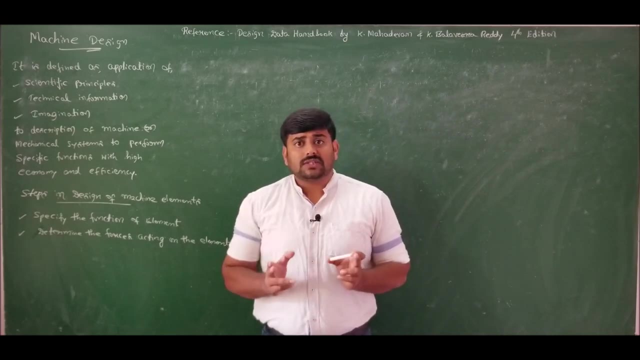 So therefore, we should determine the forces acting on the element. This force can be determined by drawing free body diagram. If I draw free body diagram, I can get the magnitude and direction of various forces on the machine element. That is hard. That is what we should be doing. 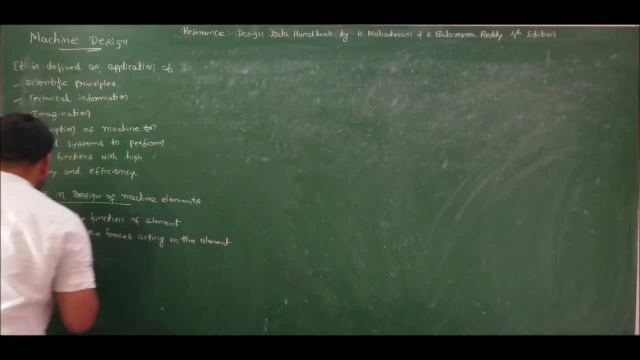 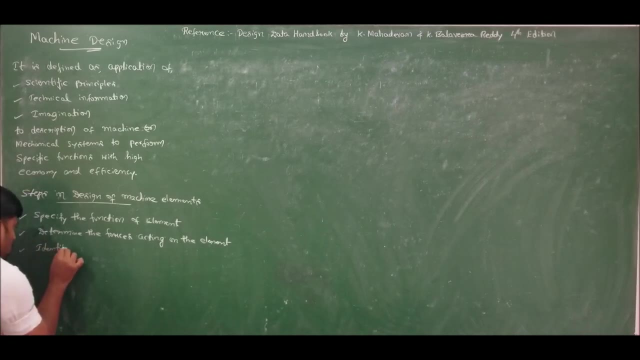 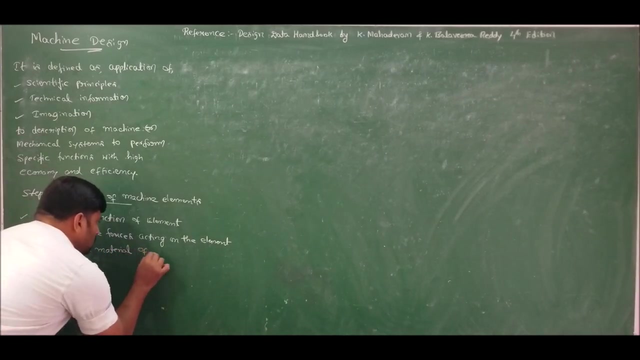 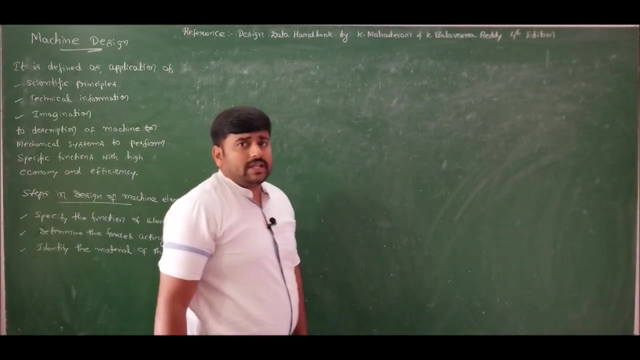 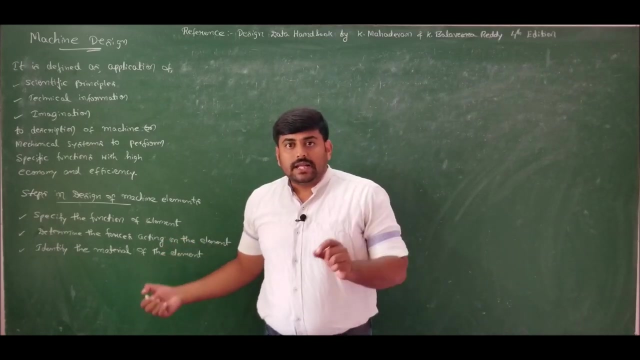 do in our second step. In the third step we should determine the suitable material for it, Identify the material of the element. Identification of material of the element is very, very important because when I am designing the machine element for fatigue loading case, then the material should possess high fatigue strength. 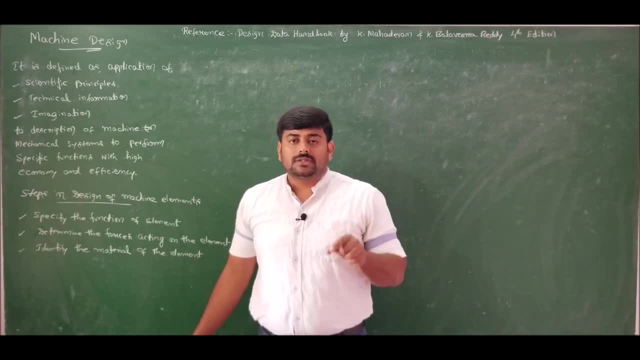 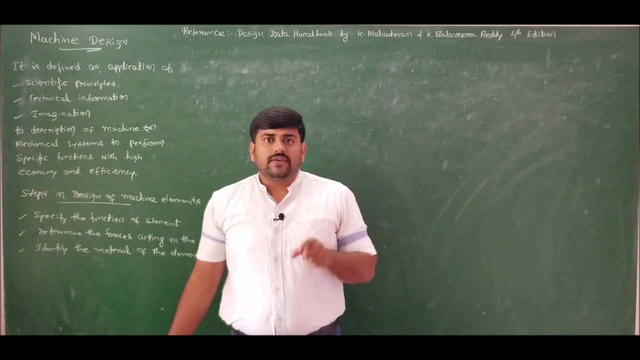 Example: chromium nickel steel has high fatigue strength, So therefore for fatigue loading applications I should go for chromium nickel steel. Similarly, for flywheels, gears, etc. we will go for casting with cast iron, because intricate shapes or difficult shapes can be. 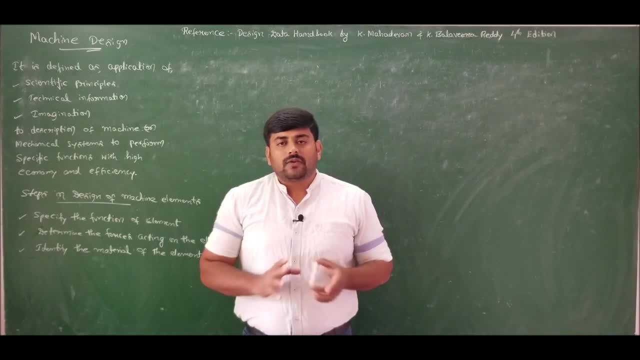 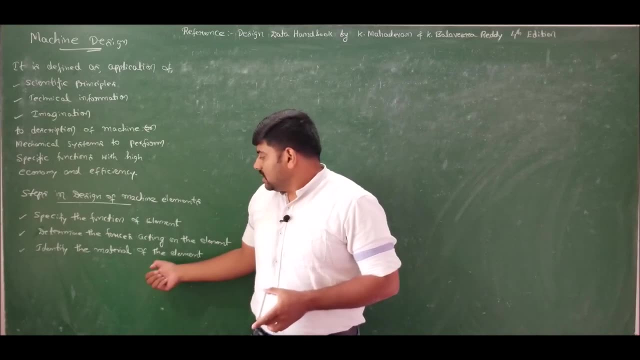 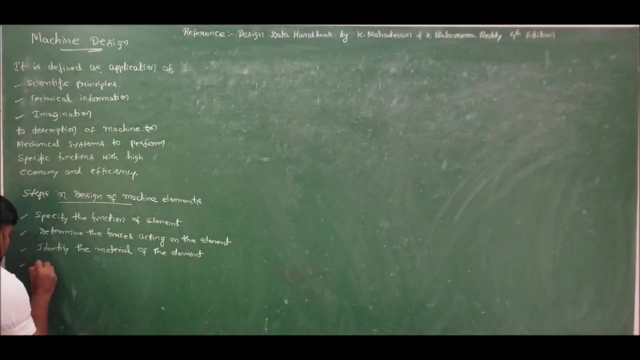 easily modeled with less machining, operation, with the help of casting. So therefore, depending on the forces, what is acting on the machine element, we should decide what material that the element should be made of. Next, the third step is the determined mode of failure. 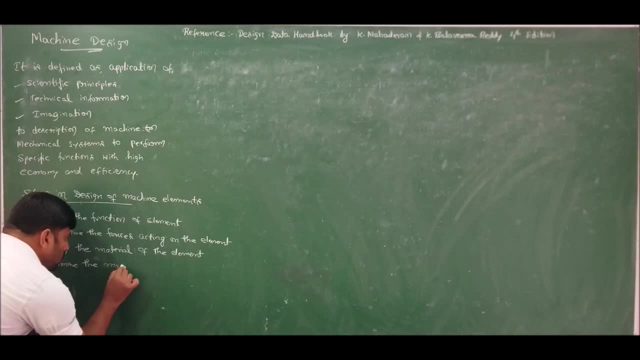 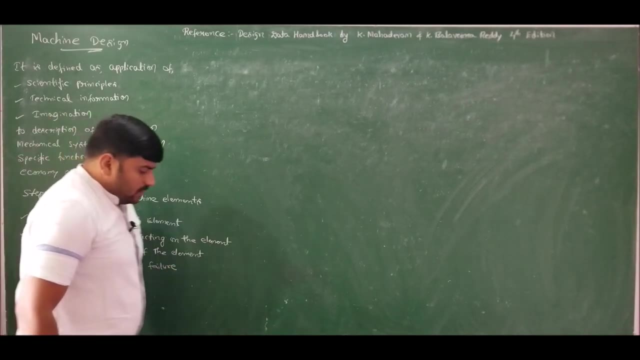 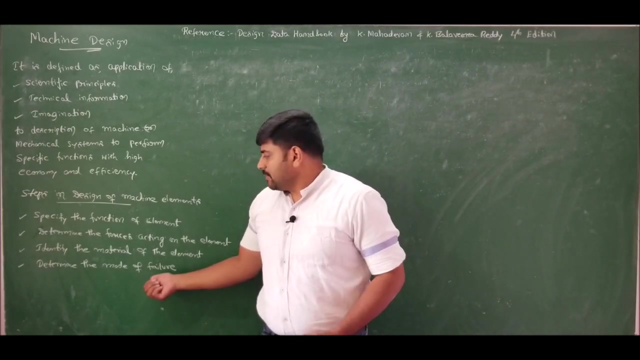 Determine the mode of failure. This failure mode might be because of Ilion, IlionAAAA yielding or because of fracture. we should determine in what mode the failure is occurring. in case of ductile material, failure occurs in cup and cone arrangement, whereas in case of 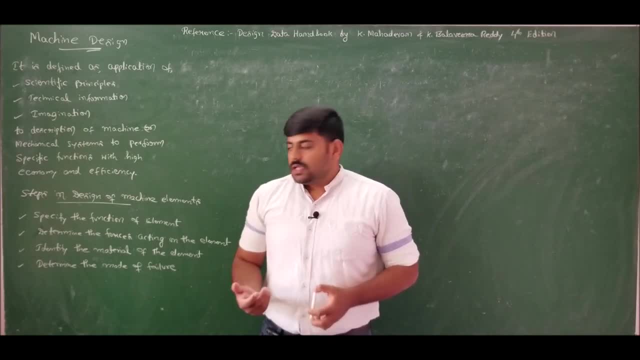 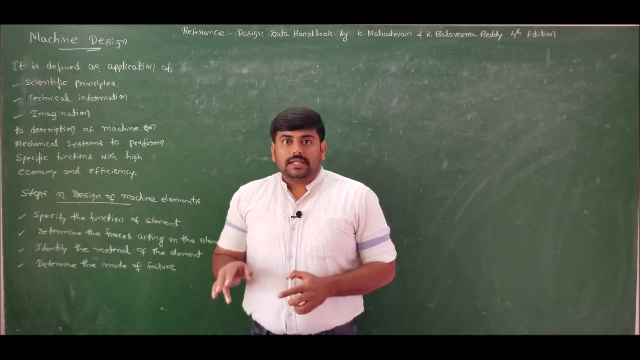 fatigue loading, it might be subjected for fracture. so therefore, we should identify what mode of failure is the machine element is subjected for, likely mode of failure. i am not telling what mode of failure the machine element is going to occur. i am telling about the likely mode of failure that 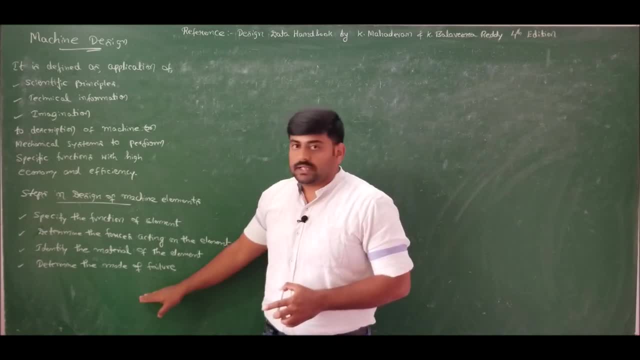 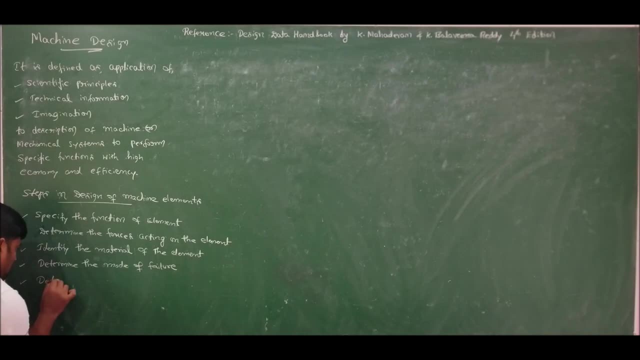 the machine member can be subjected to should be identified here, based on which i will determine the dimensions of the element. determine the dimensions. next step is to determine the dimensions. determine the dimensions of the element. like if i am designing a key, then i am interested to determine what is the width. 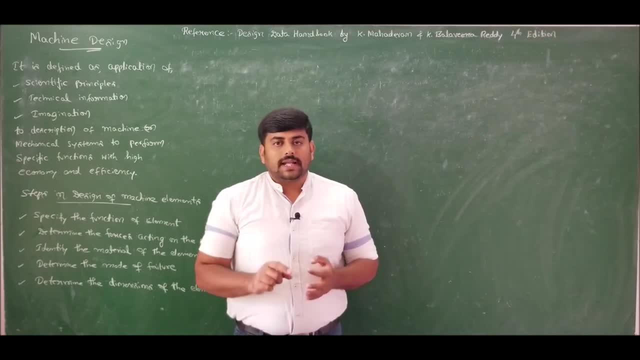 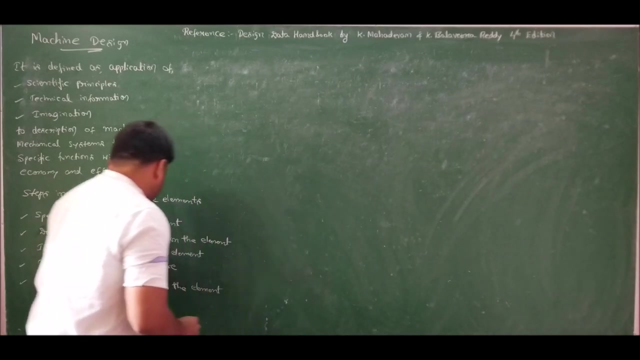 height and length of the key for connecting between the shaft and hub. if i am designing a shaft, i am interested to know what is the diameter of the shaft that is required to transmit the given power and torque. so, likewise, determine the dimensions of the element. next step: 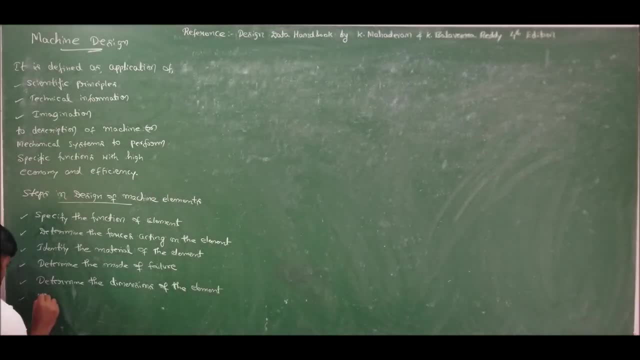 you should determine the dimensions of the element. next step is to determine the dimensions of the element. next step is to determine the dimensions of the element. next step is to determine the dimensions, которое is to modify. modify the dimensions. modify the dimensions according to manufacturing need, according to manufacturing, according to manufacturing. 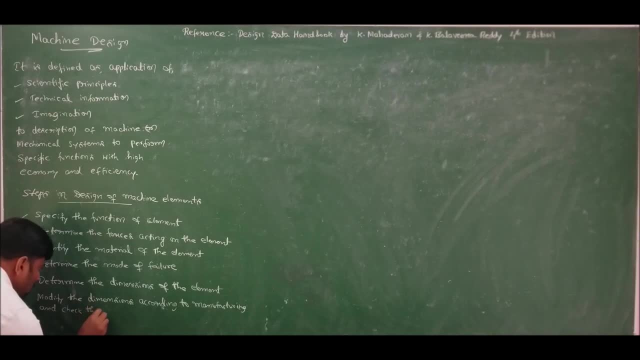 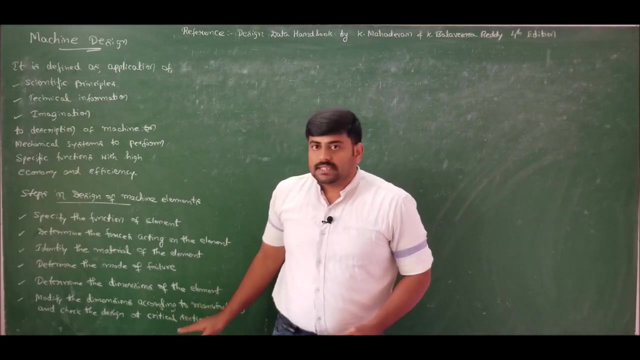 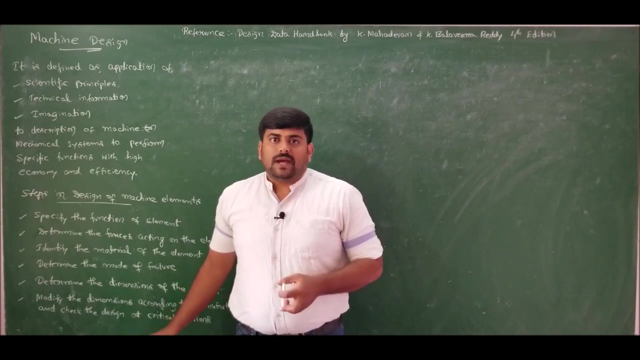 and check for critical sections and check the design at critical sections. what does this mean? once i determine the dimensions of a machine element, i should modify these dimensions. this means that if i provide shoulders, i should replace it by fillets, because shoulders create accumulation of maximum stress, termed as stress concentration. 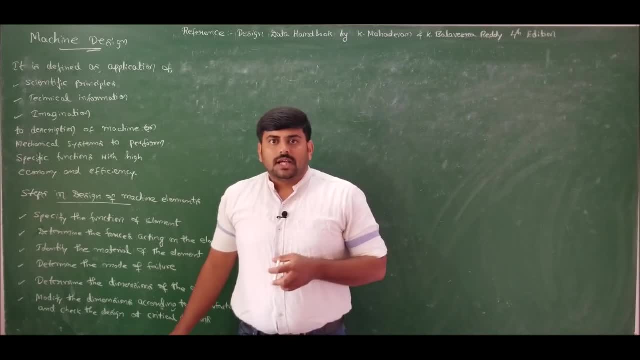 in order to avoid stress concentration, i should provide shoulders. if i have a larger role. i want to provide multiple holes in order to uniformly distribute the flow lines, such a way that the accumulation of maximum stress won't takes place around the hole which acts as a stress riser. so 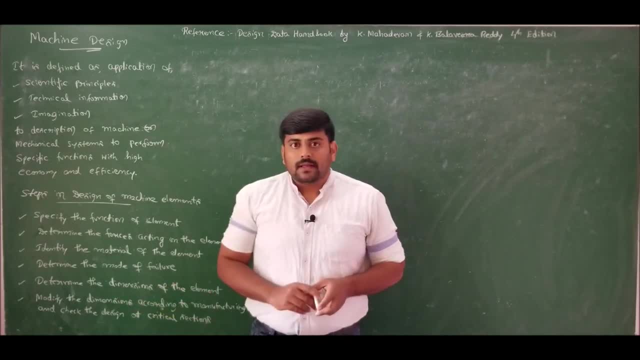 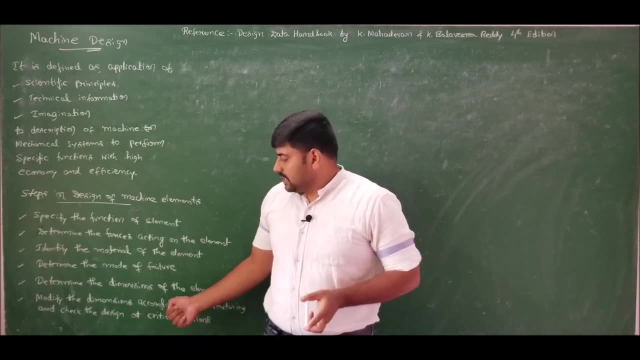 therefore, we should modify the dimensions according to the manufacturing requirement and also we should analyze you these. the modifications cause any changes lead to the failure of this specimen or not, or failure of the machine element or not. therefore, we should recheck the design for critical sections once. 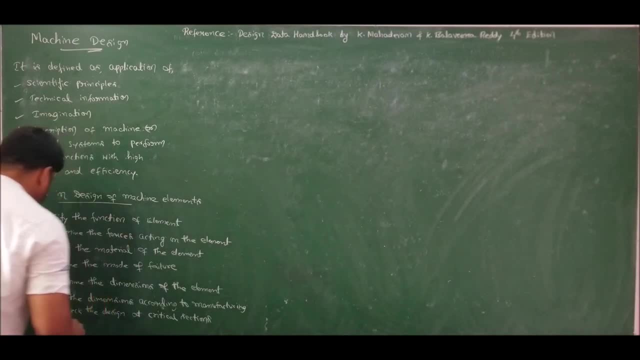 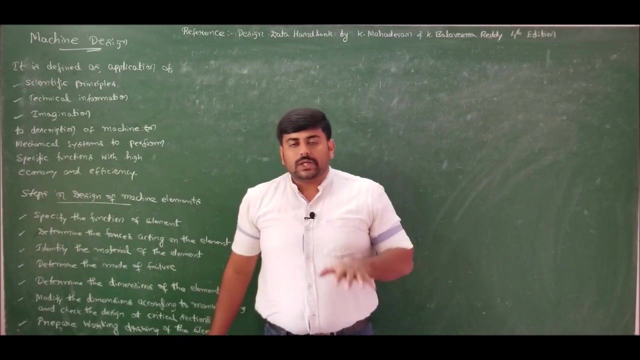 all these steps have been done. finally, we will prepare the working drawing of the element. so finally, we'll come up with prepare working drawing. so finally, we'll come up with prepare working drawing of the element. so, in the final step, we are going to prepare the working drawing of the element. this. 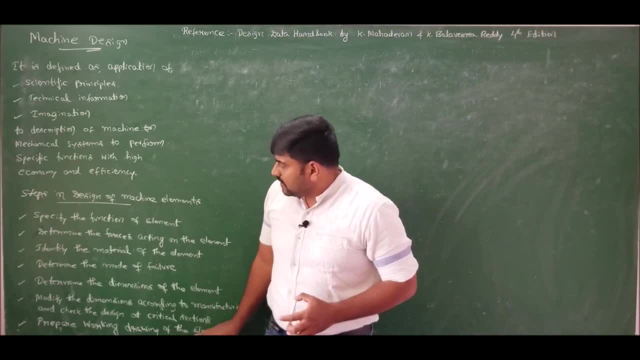 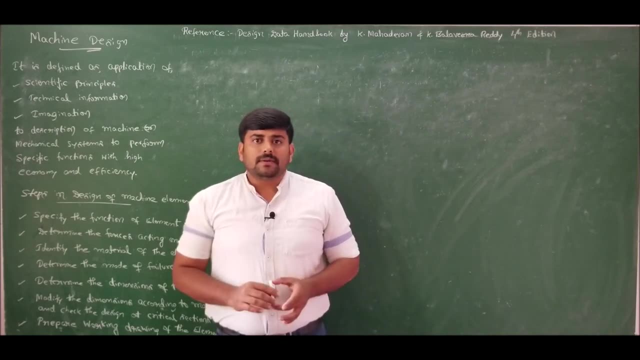 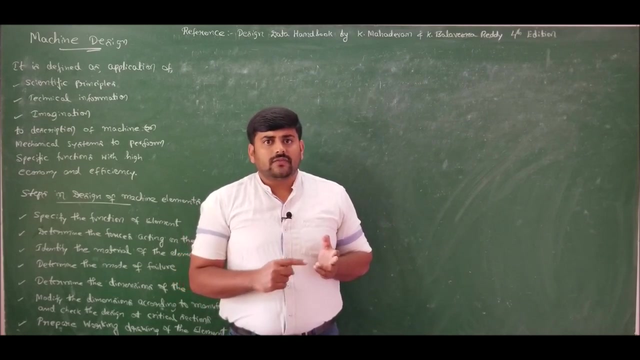 working drawing of the element contains the tolerance, fits, dimensions. what are the various design of machine element? So in this course we will be addressing various machine members and we are going to design various machine members. like we are going to determine the dimensions, we are going to analyze the various forces acting on them. Since this course is very 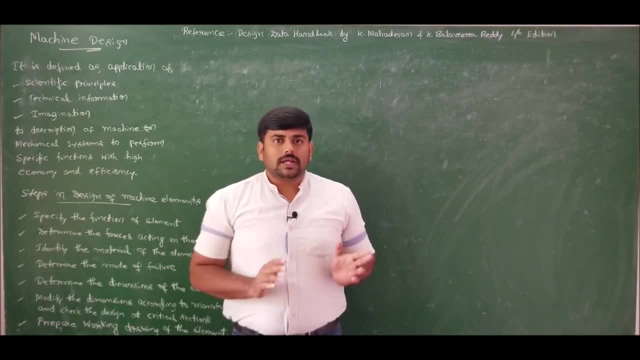 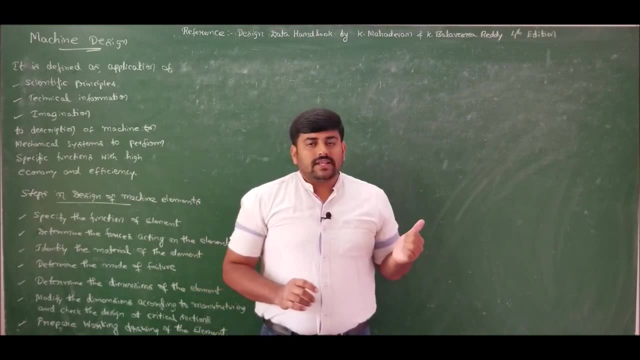 vast. I am dividing this machine design course into two parts: design of machine elements 1 and design of machine elements 2.. I am going to address in the final part of today's lecture what I am going to take up in design of machine elements 1 and what I am going to address in the 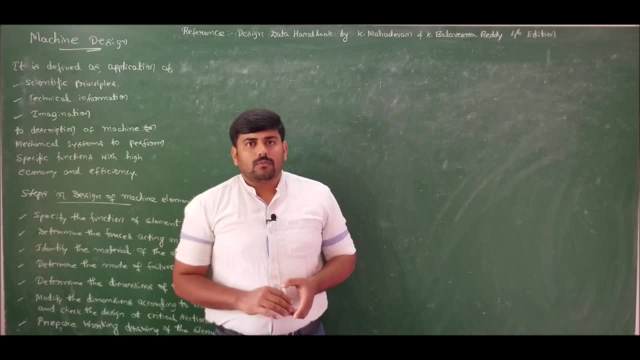 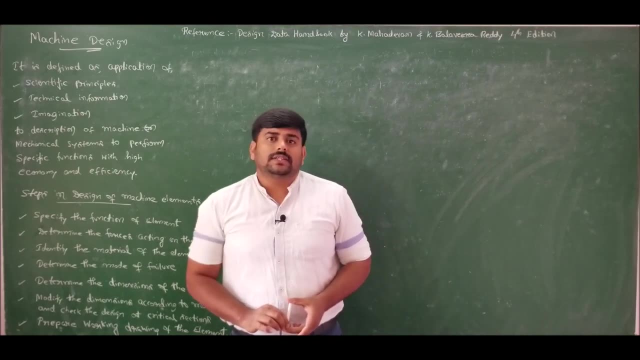 second part, that is, design of machine elements 2.. Before moving for the syllabus of this course, I am interested to address the various properties of engineering materials We have learned. what is the meaning of machine design? what are the steps involved in design of machine element? and next is: 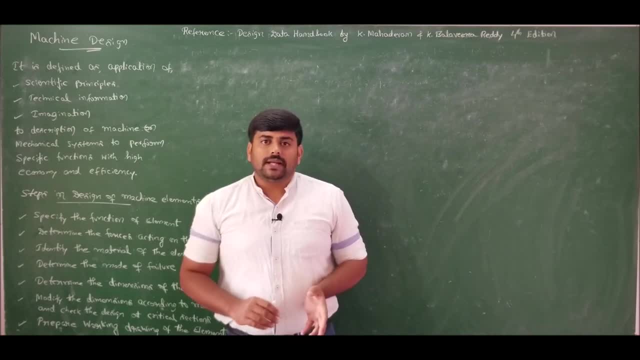 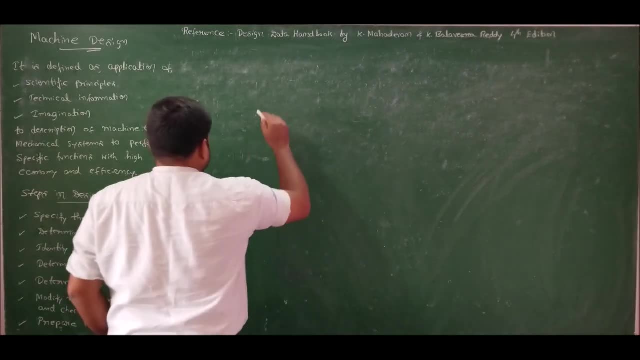 materials. Material is very, very important. So selection of material is based on the mechanical properties of the material. So selection of material is based on the mechanical properties of engineering material. The important mechanical properties that one should know in design of machine element is first one. So next we are discussing about properties of engineering. 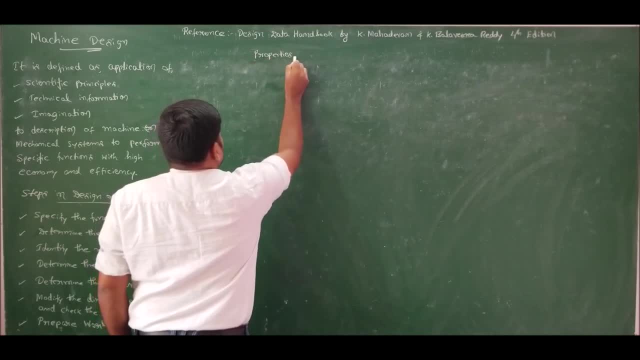 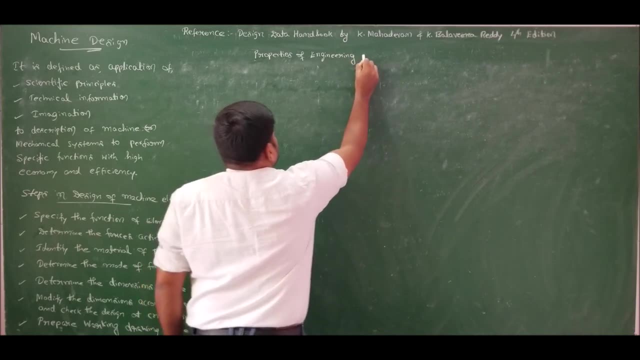 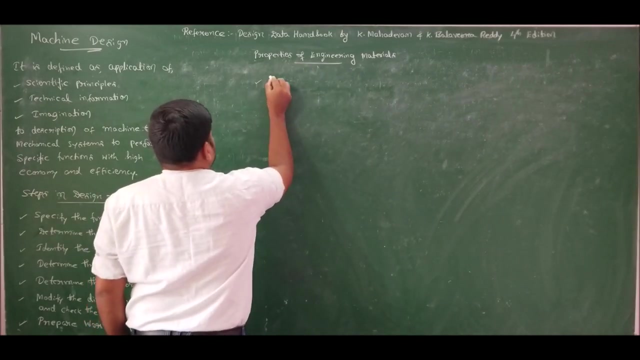 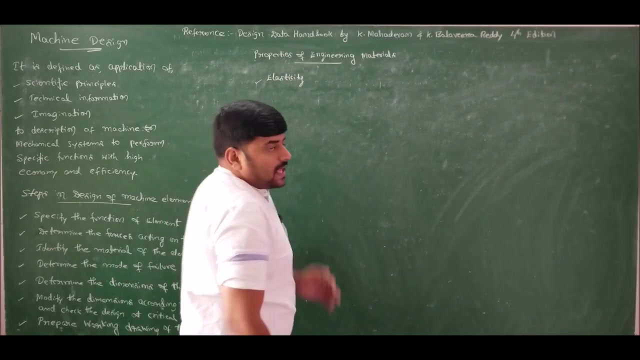 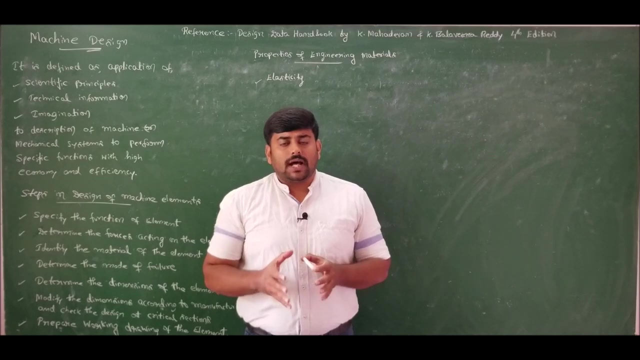 materials. Properties of engineering materials. First one is engineering materials. So engineering materials are costing chemicals in a condition which is not the most of the market, because there is no way that communications, cooperation and localization takes place without correct health, proper maintenance, operational activities and quality If such infrastructure 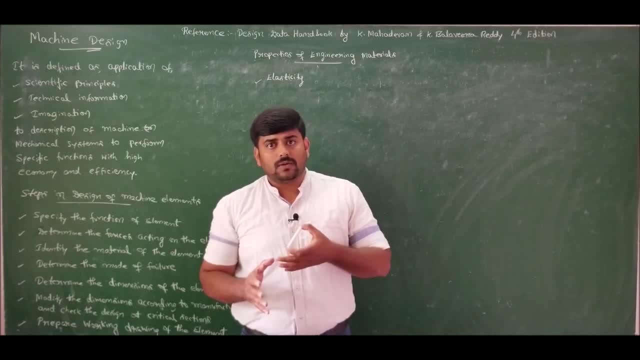 is available. communication with legitimate manufacturers has the perfect ability to provide a good system using real-world interface, key features systems, as well as Glück, Heart, onnenhire to make the absolute best microwave revolution. This means, however, inexplaining materials is not sufficient for the malformatism aspect of engineering. Denote another point which is 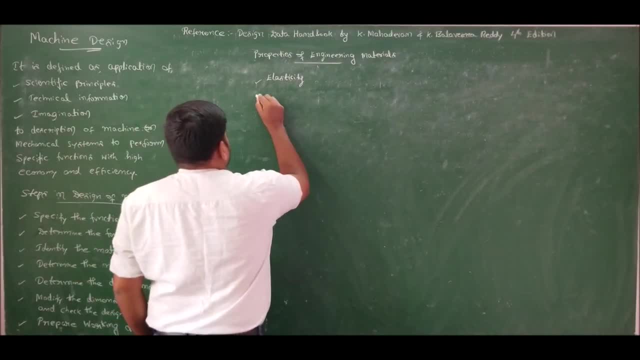 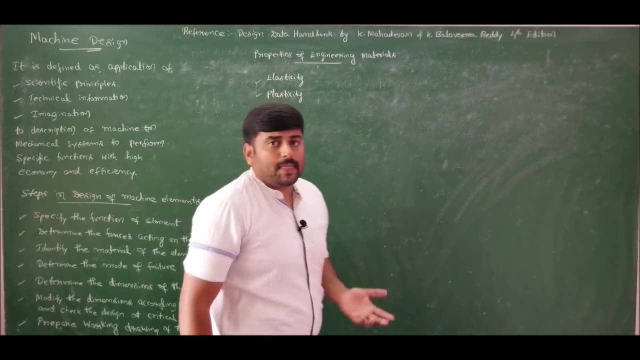 important. When we say the material starts essentially from floor material to floor material, the material experts understand it. So how we can change it. In the général this is known as elasticity. second property is plasticity. plasticity is opposite to elasticity, in which the material will deform under the 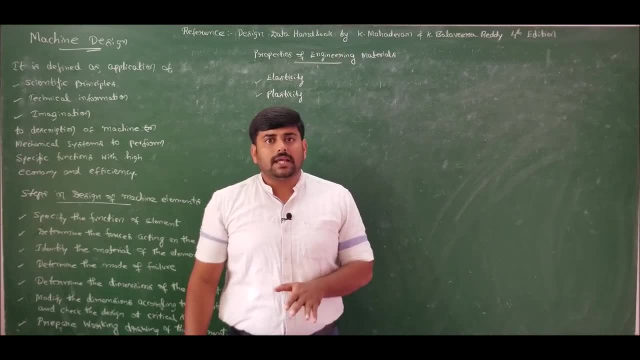 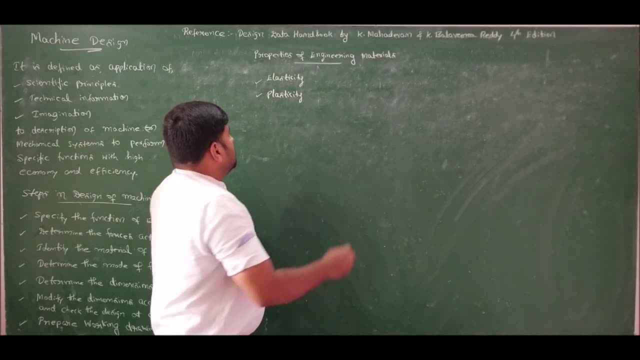 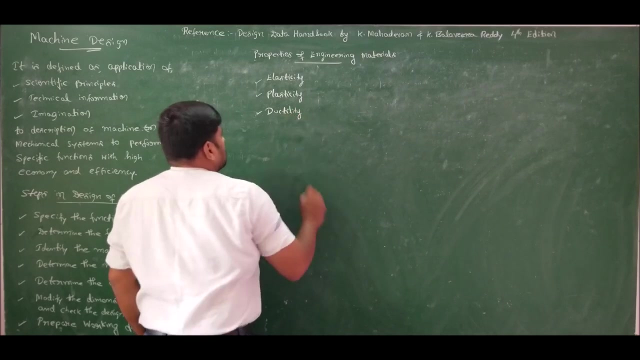 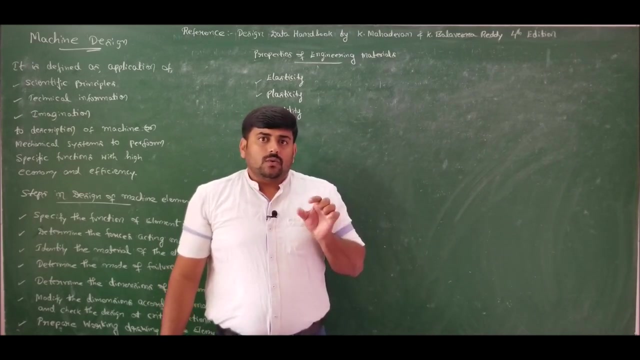 application of load and retains the deformation permanently, even though we remove the load later. so therefore, plasticity is the opposite to elasticity. next mechanical property one should know is ductility. ductility is defined as the ability of a material which can be drawn into thin wires, that is, ability of a 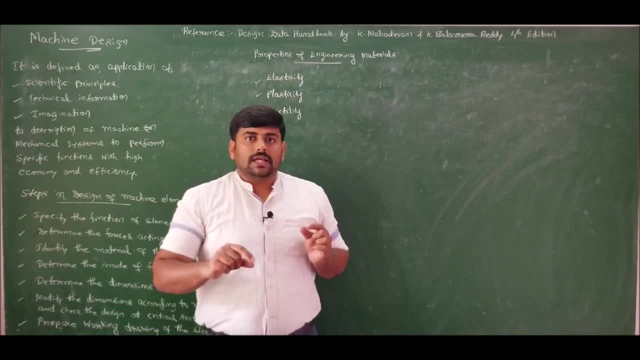 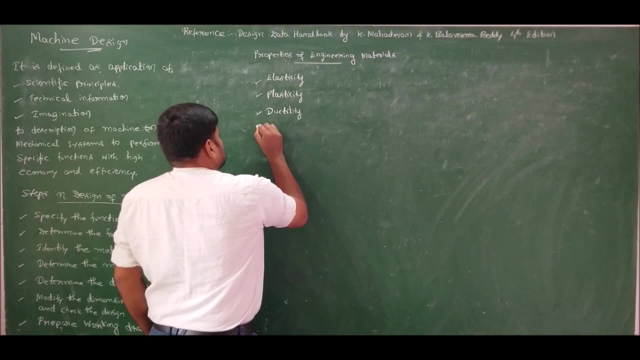 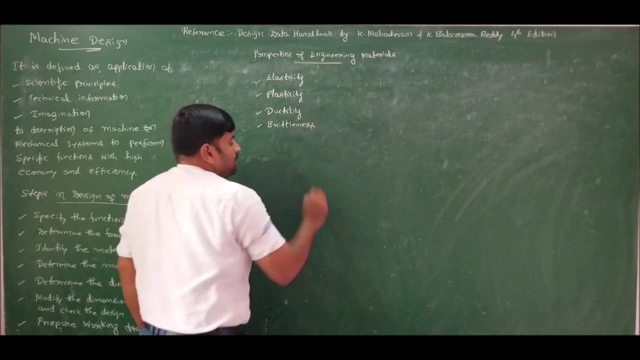 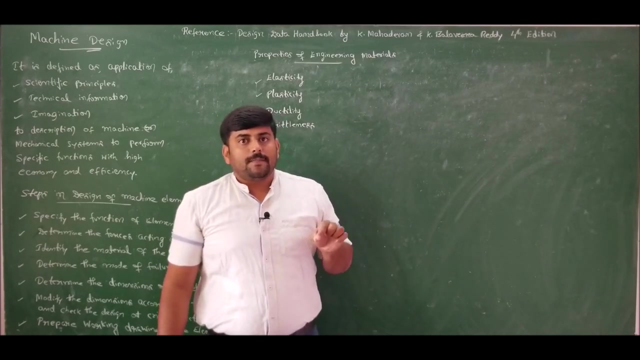 material to deform in the longitudinal direction under the application of tensile force that is drawn into thin wires, whereas the opposite to ductility is brittle. brittleness is opposite to ductility, where in which material cannot be drawn into thin wires or it will not deform longitudinally under the application of. 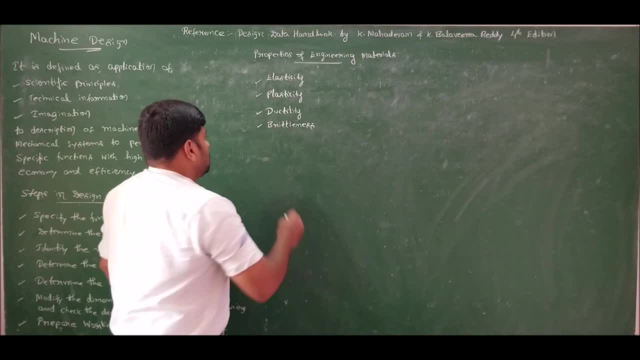 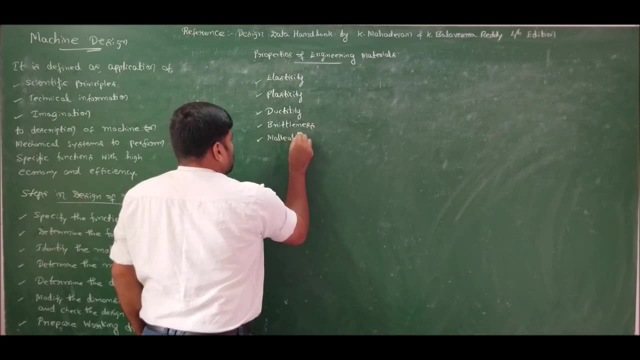 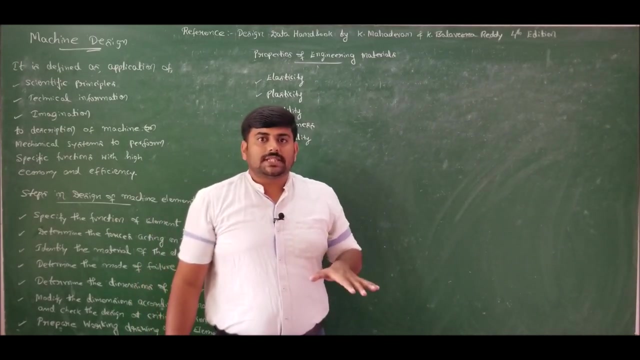 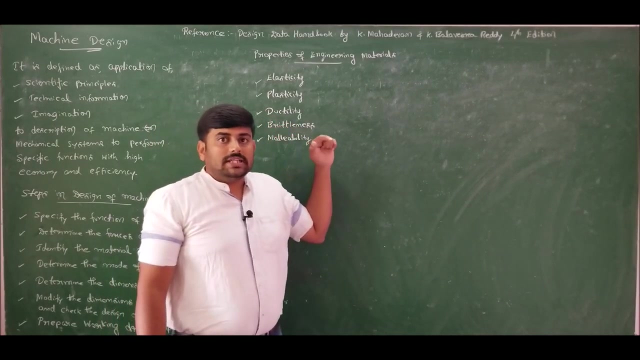 tensile force is termed as brittleness. next we have malleability. malleability is the property of an individual material which can be drawn into thin sheets in which the material can deform in all the directions, whereas in case of ductility, material will deform only in the dog longitudinal direction under the 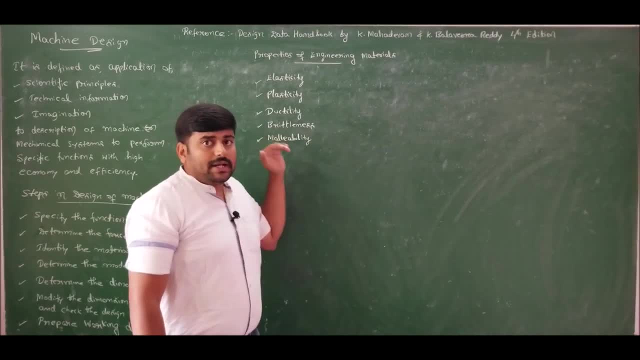 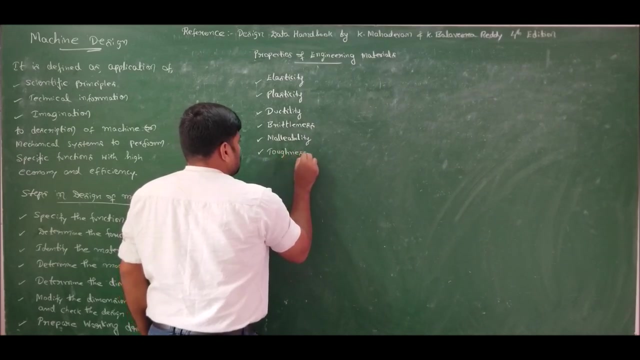 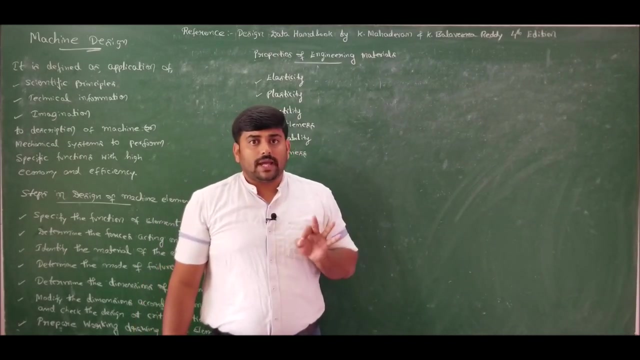 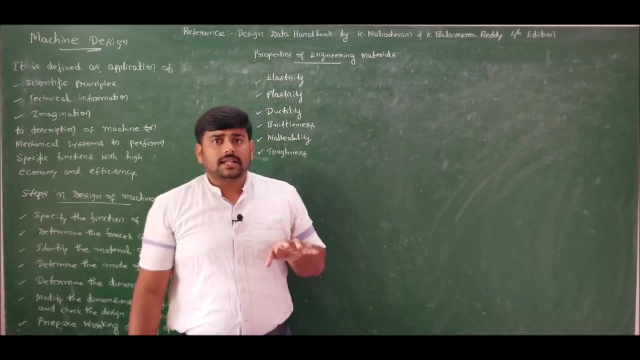 application of tensile force, whereas in case of malleability, material will deform in all directions, where in which it can be drawn into thin sheets. next engineering property of material is toughness- toughness. toughness of an material is defined as the ability of a material to absorb energy until fracture. the ability of a material to absorb energy until it. 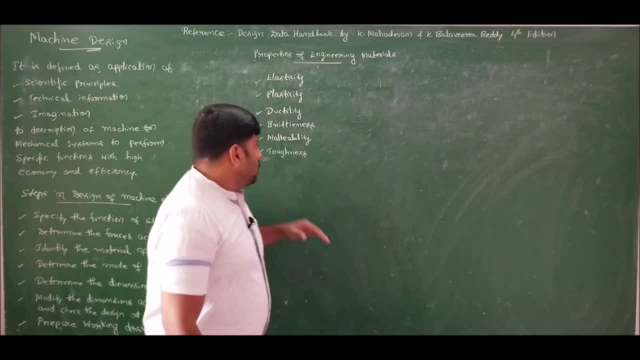 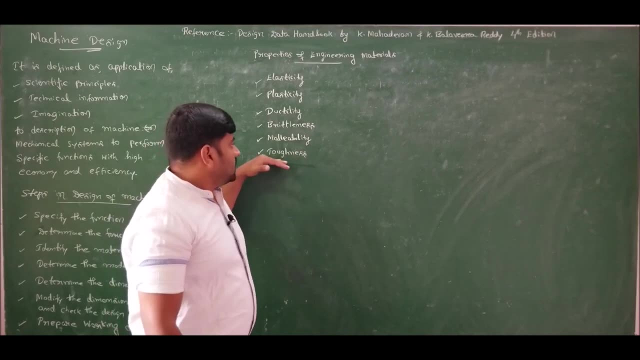 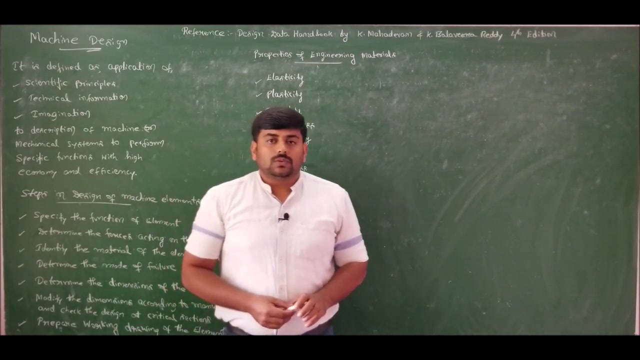 gets fractured or break down. so the amount of energy absorbed by engineering material until it is get fractured, that is termed as toughness. next engineering property is hardness. hardness is defined as the ability of an material to withstand surface abrasions or surface indentations. the ability of a material to resist surface abrasions or surface indentations. 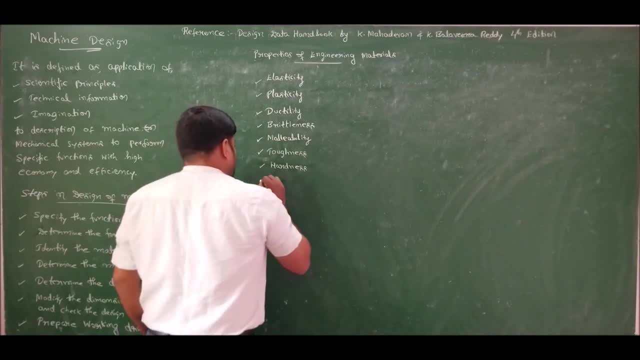 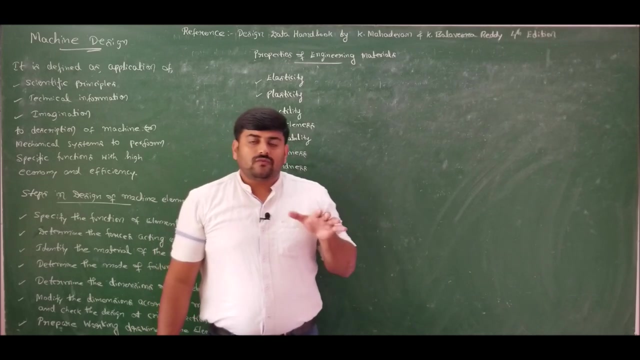 is termed as hardness. next property of engineering material is stiffness, stiffness. stiffness is defined as the amount of force required to produce unit deformation staring machine that never expires. so stiffness is generally defined as Salesforce required to produce. you need to deformation, forsique, hydro produce. you need to. 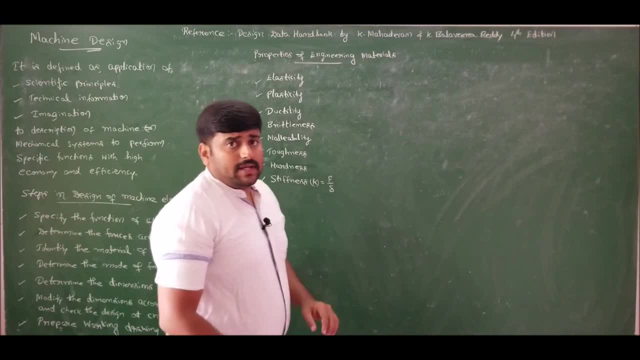 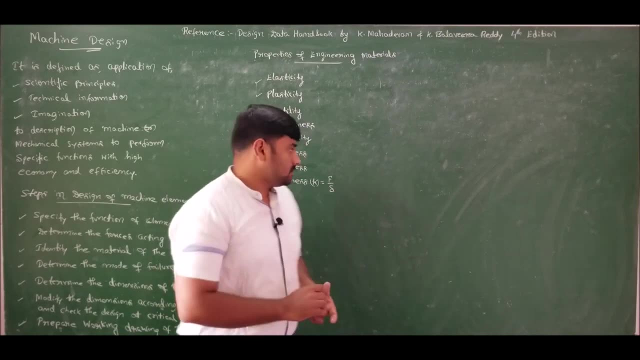 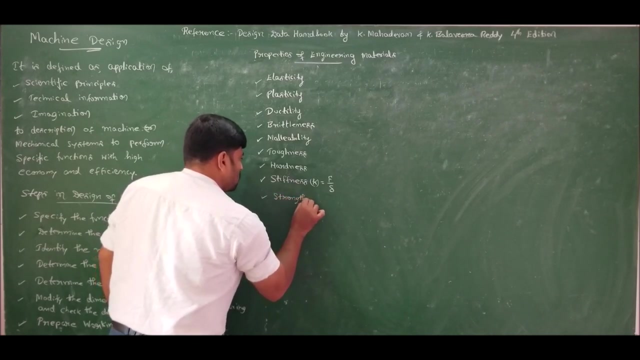 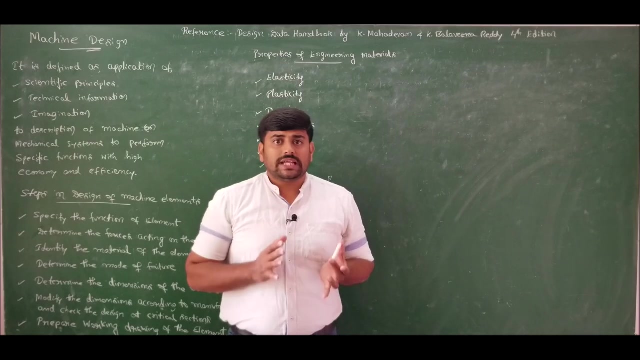 deformation is termed as stiffness. in engineering materials, it is measured to deal of models of elasticity, whereas stiffness is a very, very important property for springs. next we have strength. strength of an engineering material is defined as the ability of the material to withstand load without yielding or breaking the 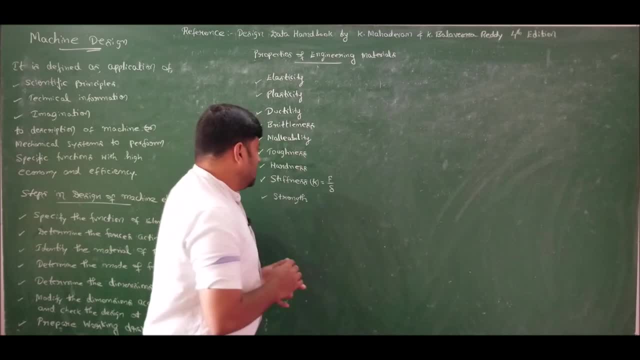 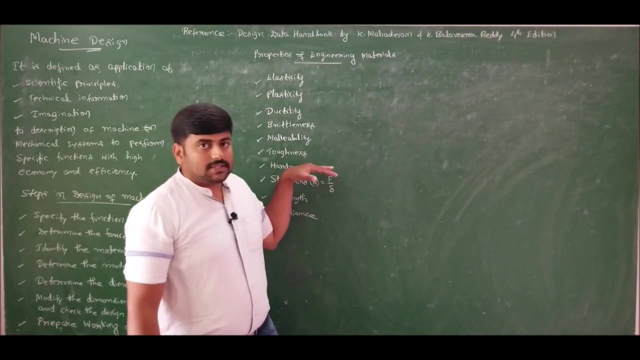 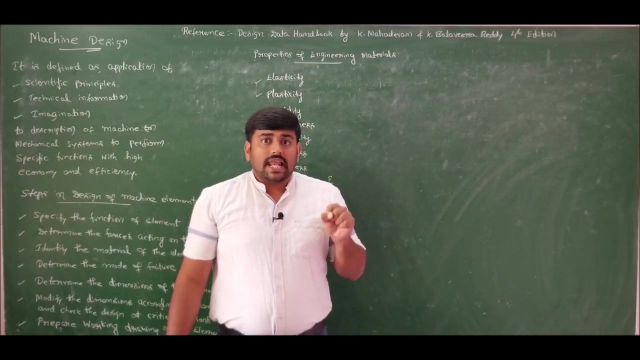 ability of a material to withstand load without yielding or breaking. next property is resilience. resilience- resilience is somewhat similar to toughness. it is also defined as the ability of a material to absorb energy within the elastic limit without yielding or breaking is termed as resilience. resilience is measured as: 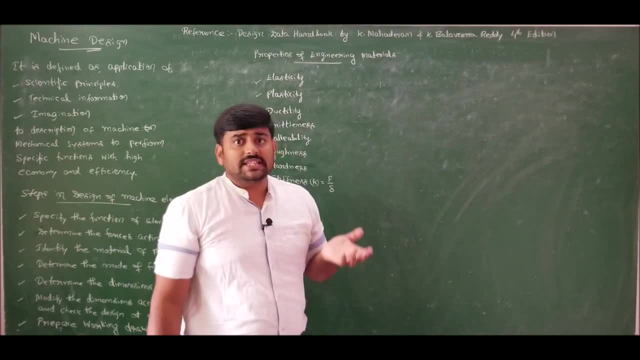 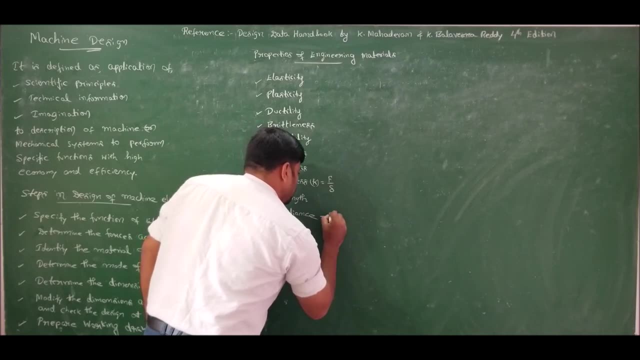 amount of energy absorbed per unit volume within the elastic limit. so resilience is ability of a metal to absorb energy within the elastic limit- this is within the elastic limit- whereas toughness is ability of a material to absorb energy until fracture- until fracture. so this is a difference between 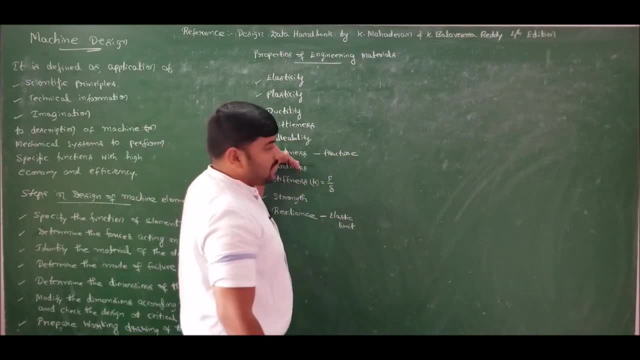 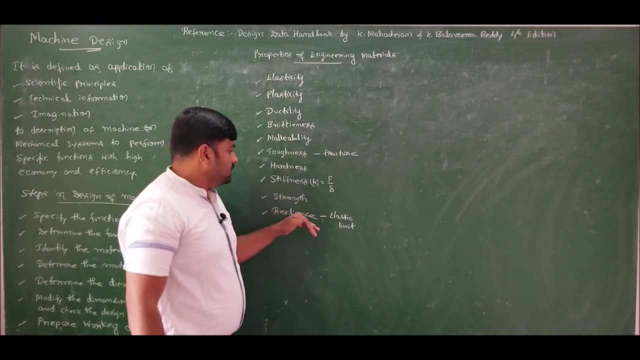 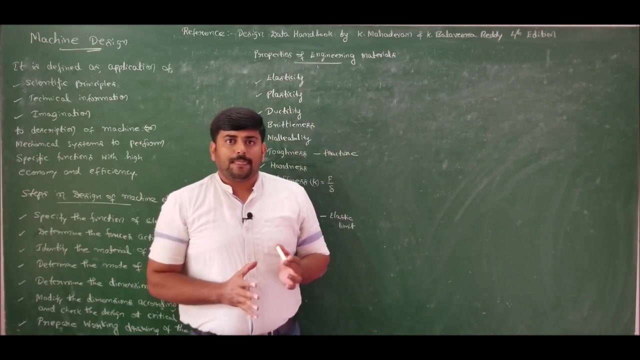 resilience and toughness. resilience and toughness are the ability of material to observe energy when it is loaded or when it is subject for impact or shock. this is measured until elastic limit, whereas this is measured until fracture or failure. next important property is creep. creep is defined as when a material is subjected for high temperature, constant stress. 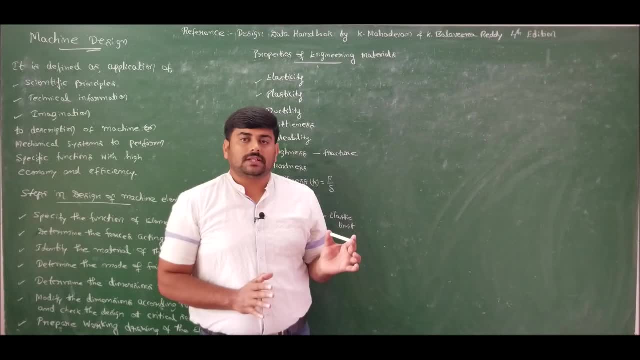 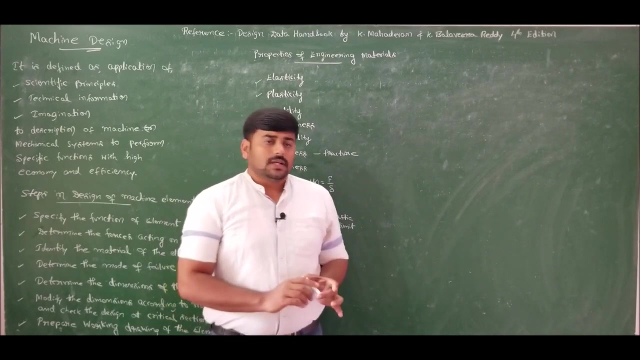 for a longer duration, the material undergo permanent deformation, which is termed as creep. i repeat: when an engineering material is subjected for constant stress at high temperature for longer duration of time, it will undergo a permanent deformation, which is termed as creep. example for creep effects are turbine blades. 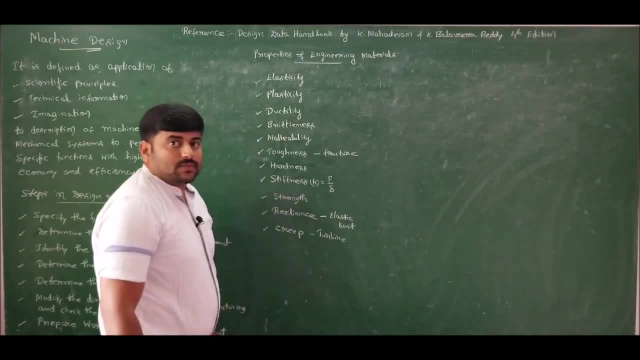 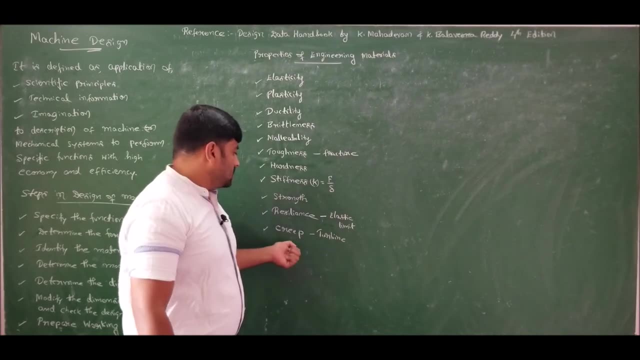 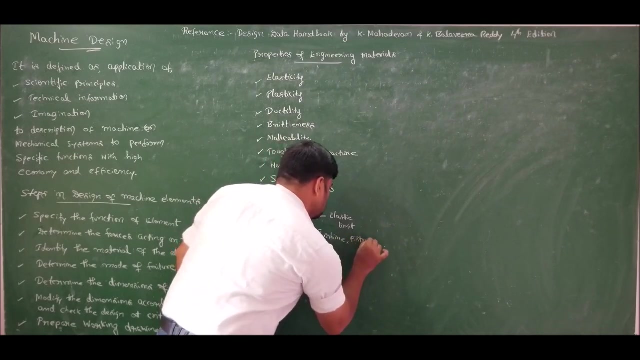 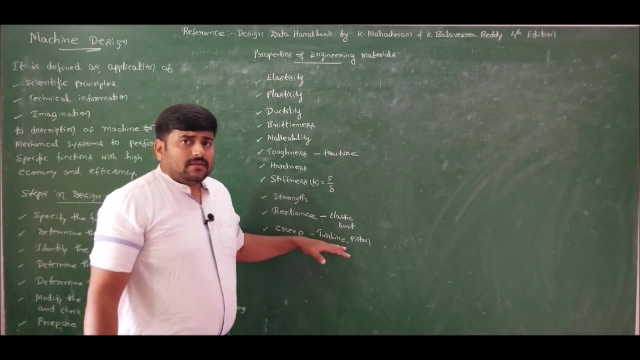 steam turbine blades which are subject for constant stress at high temperature for longer duration of time, which will undergo a permanent deformation which is termed as creep and creep piston ice engine. piston ice engine connecting rod. these are an example for materials or mechanical machine members which are subjected for creep effects. so these are some. 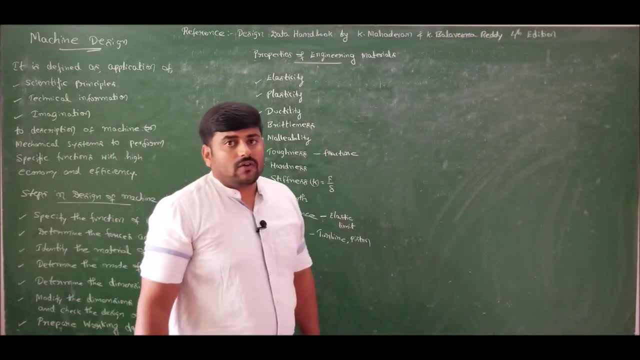 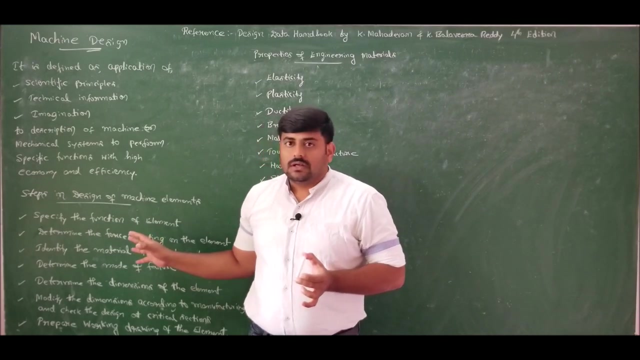 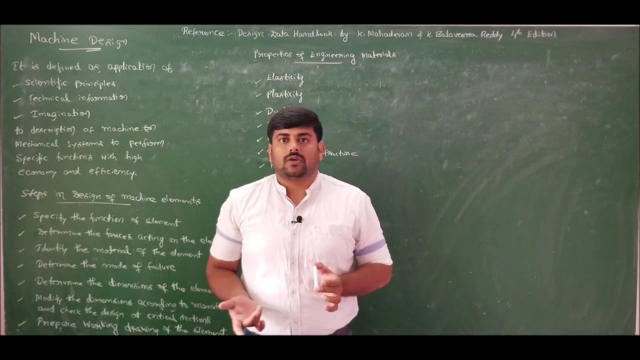 very, very important mechanical properties of engineering materials which one should know. and if you are well aware of these mechanical properties, you can choose the proper engineering material for the specified application and we can design the machine element in order to perform the specified function with high efficiency and high economy. 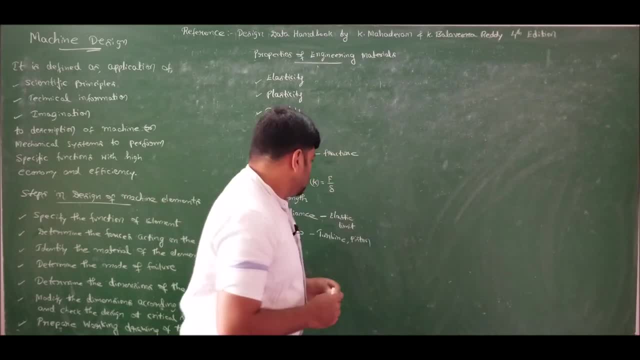 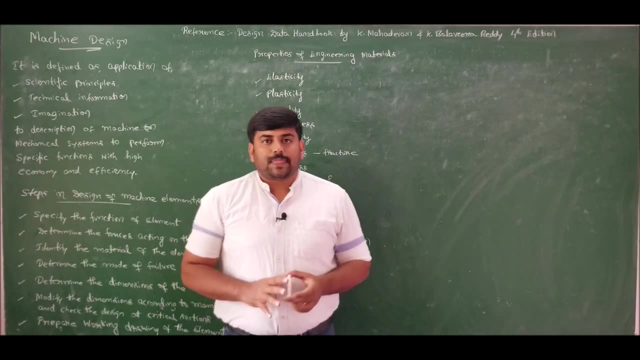 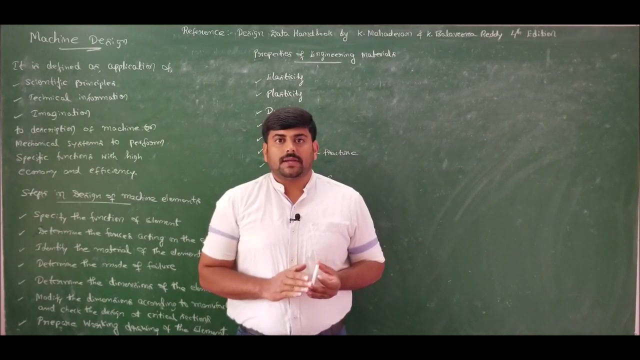 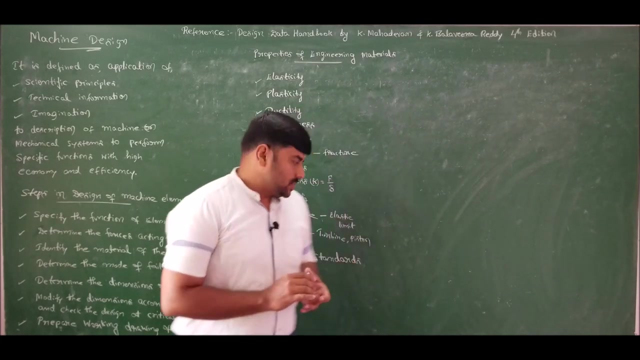 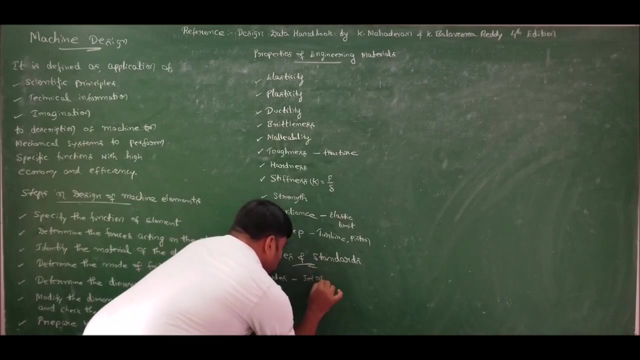 now moving ahead, let me discuss about codes and standards. codes, codes are defined as set of specifications for design, analysis and fabrication or manufacturing intended to have high degree of safety, efficiency and quality. so codes are defined as. codes are defined as set of specifications for set of specifications for design analysis. 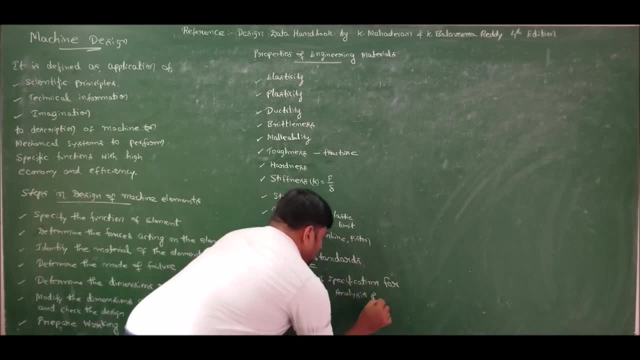 so codes are defined as set of specifications for design, analysis and manufacturing intended to have higher degree of safety. why we have these specifications? the purpose is to have. the purpose is to have high degree of safety, high degree of safety efficiency and quality in order to have high degree of safety efficiency. 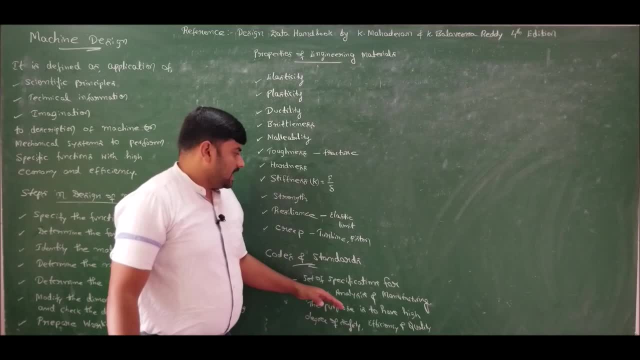 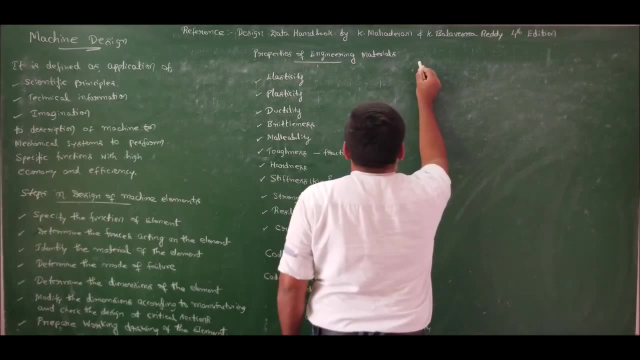 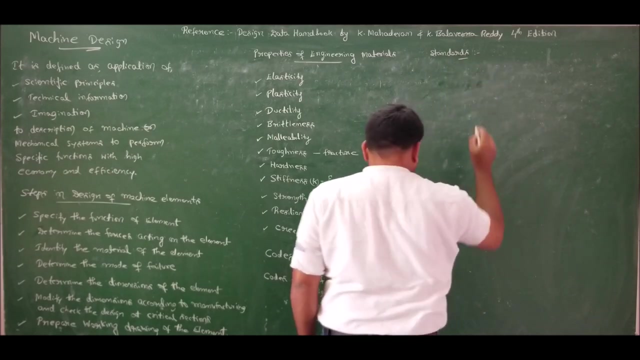 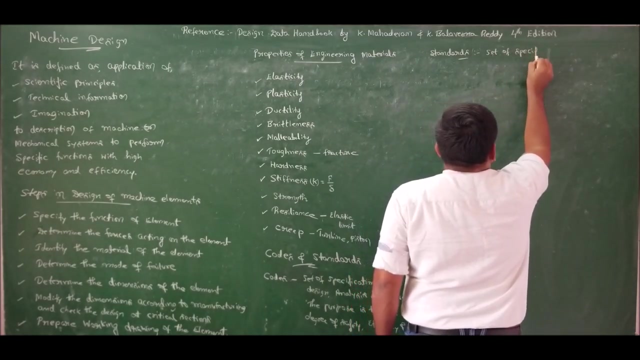 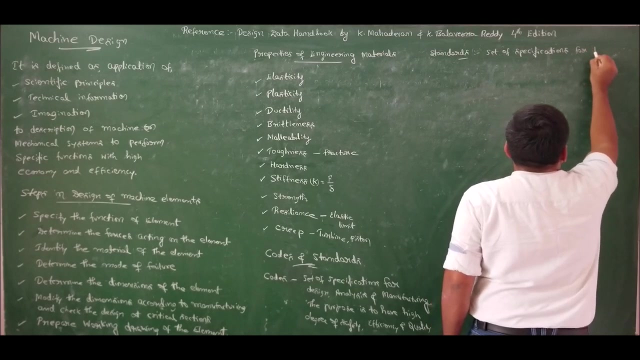 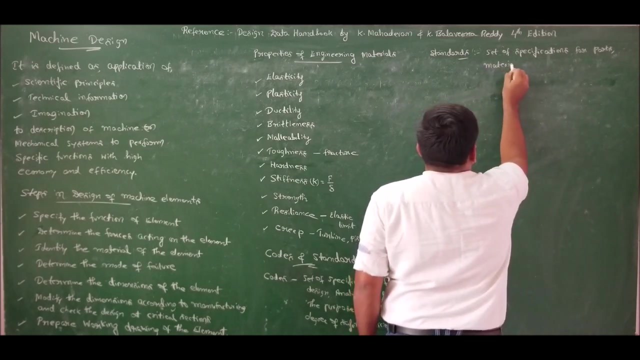 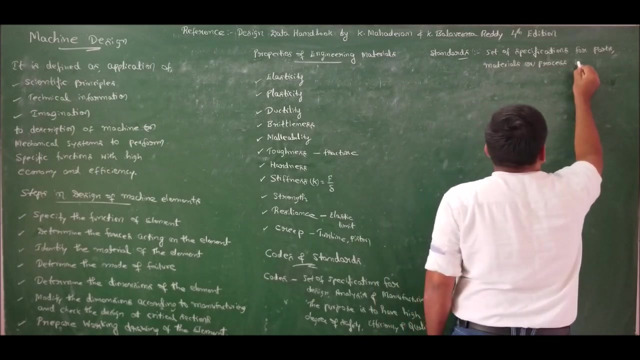 and quality. we are setting some specifications for design, analysis and manufacturing. this is termed as codes, whereas standards is defined as coming for standards. standards is defined as coming for standards. standards is defined as set of specifications, set of specifications for mechanical parts or processes, materials or processes. why we have the set of standards? we have this set of standards. 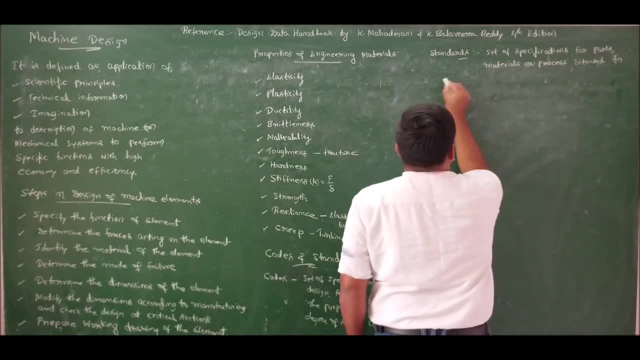 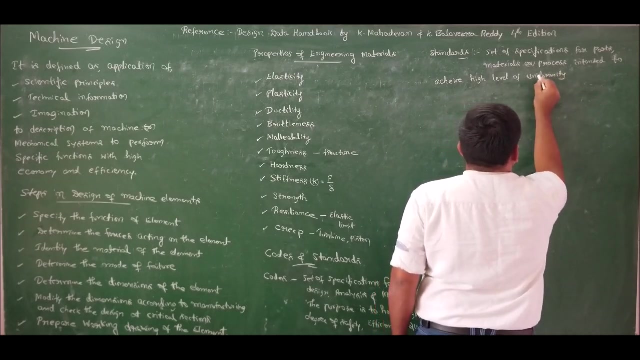 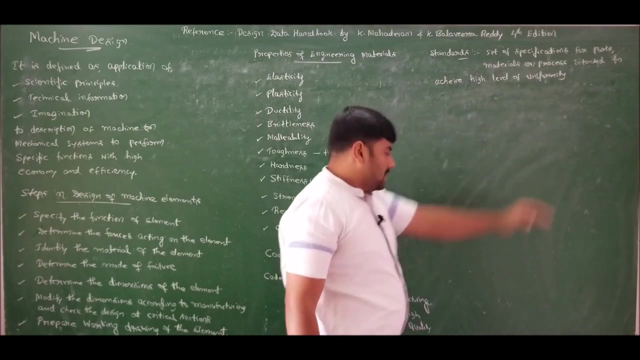 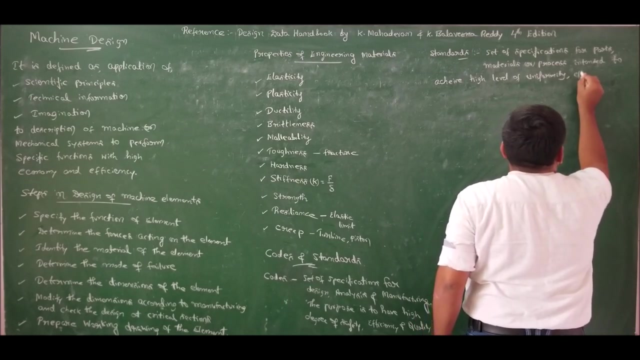 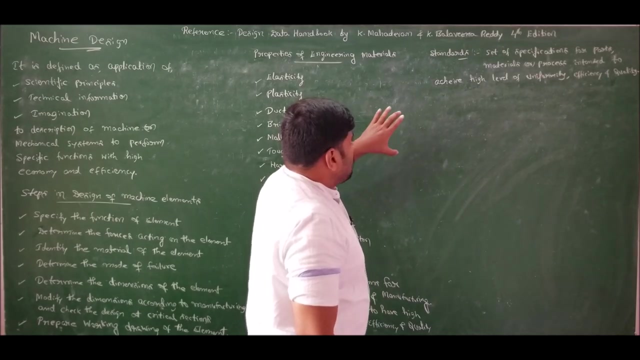 intended to achieve, intended to achieve high level of uniformity, very, very important high level of uniformity, high level of uniformity. standards are very, very important to achieve uniformity, whereas codes are important to achieve safety and then to achieve high level of uniformity, efficiency and quality. so this is about codes and standards coming for specification of 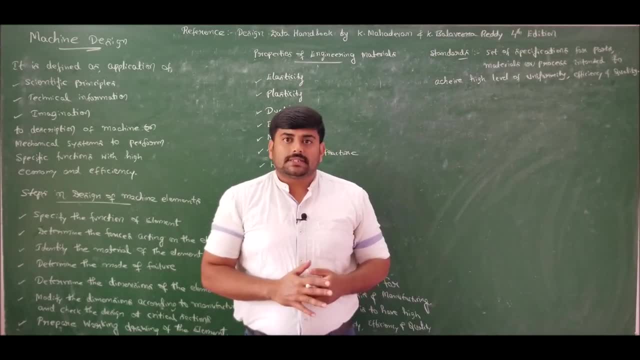 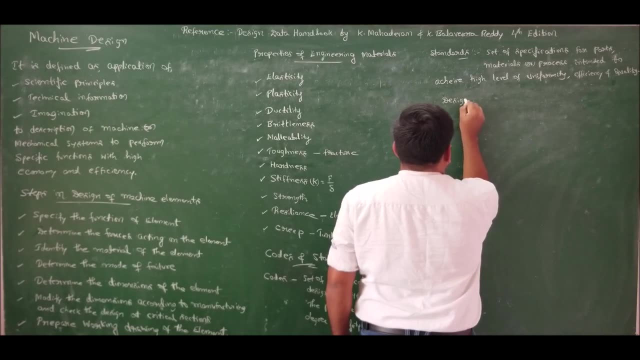 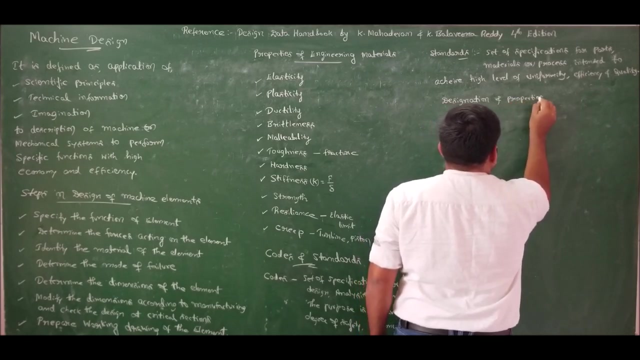 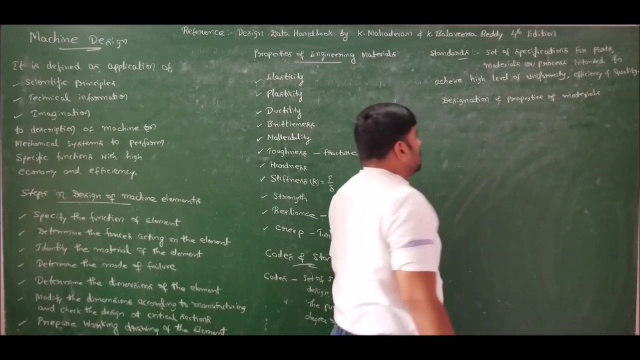 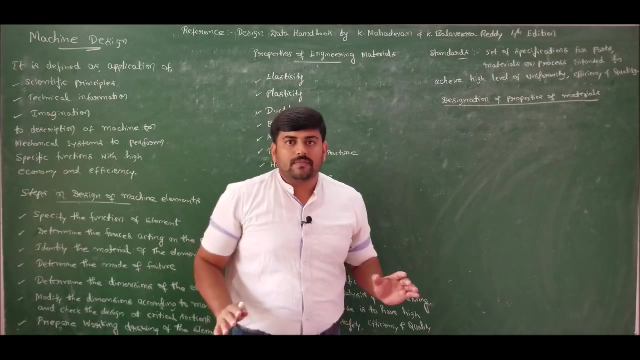 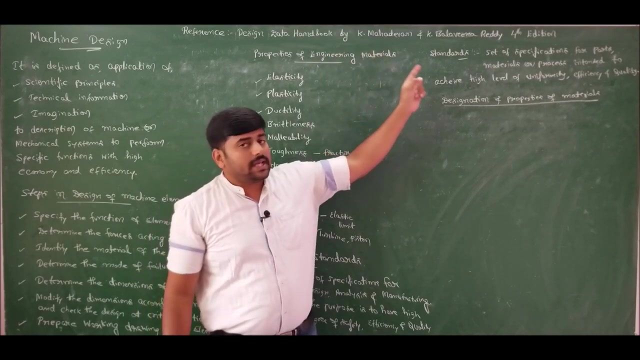 or designation of materials in engineering. coming for designation. coming for designation and properties of materials using codes and standards. we can directly refer our data handbook for this complete course on machine design. I will be using machine design data handbook- design data handbook written by K Mahadevan and K Balavir Reddy, fourth edition. I will be using this design. 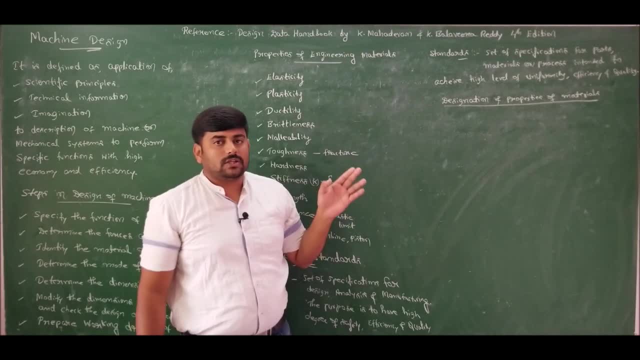 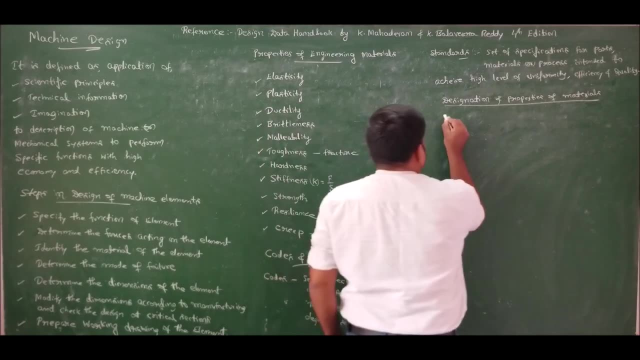 data handbook for this complete course on machine design, both for design of machine elements one as well as for design of machine elements two. in this design data handbook, if you refer, refer design data handbook. the short end of DDHP stands for design data handbook. I am using. 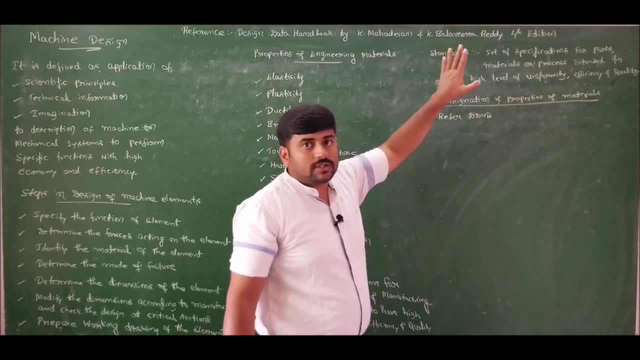 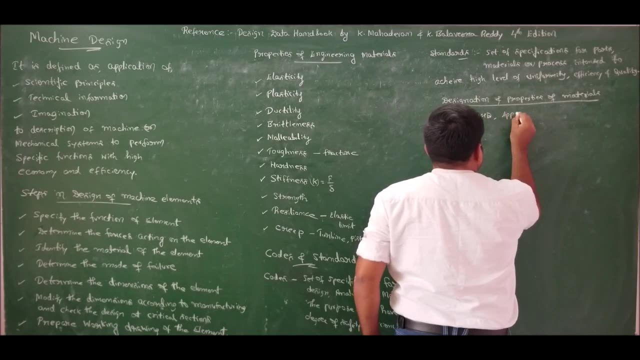 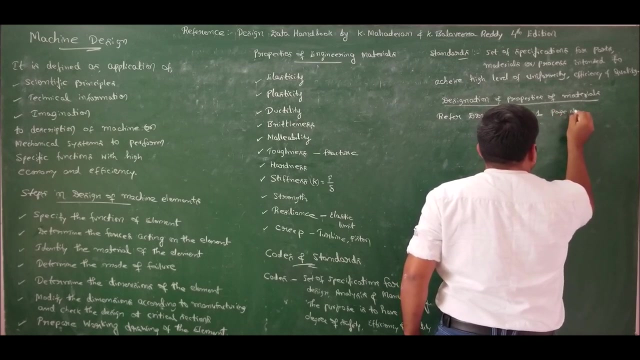 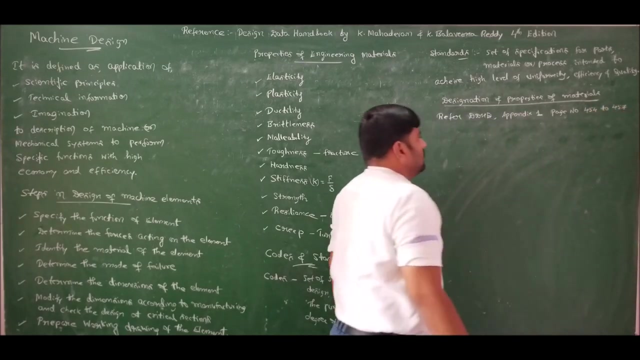 design data handbook written by K Mahadevan and K Balavir Reddy, fourth edition for this complete course. so in this book, if you refer appendix one, appendix one, that is, page number, page number 454 to 457, you have the designation and properties of materials. example: if i give Fe 350, this: 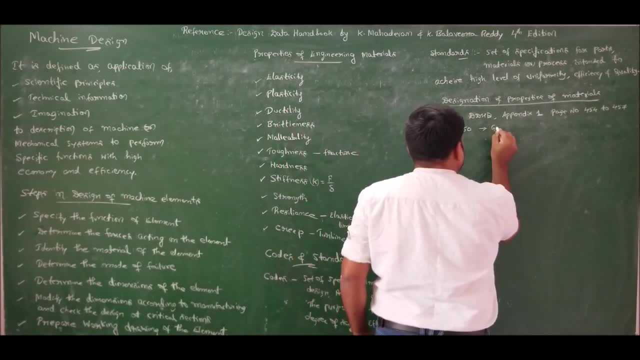 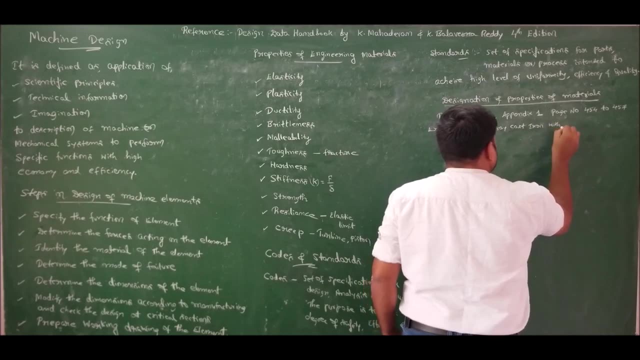 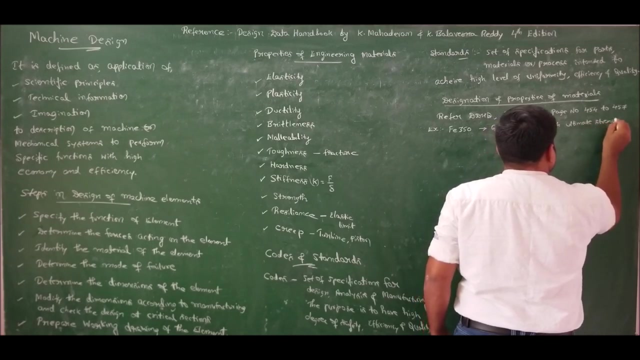 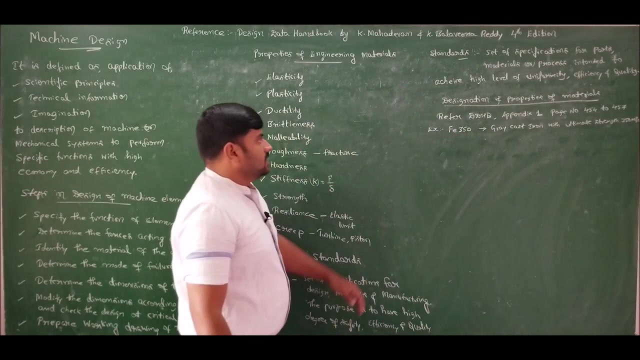 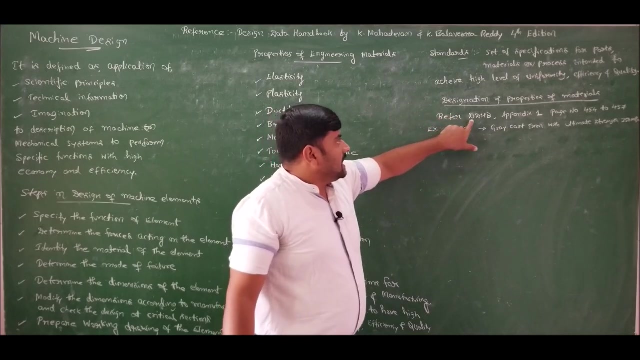 means that it is a gray cast iron. it is a gray cast iron with ultimate, ultimate, ultimate ultimate strength of 350 mpa, with ultimate strength of 350 mpa. this is what this code stands for: fe 350. like this. for various codings you can refer design data handbook, appendix 1, page number 454 to 457. 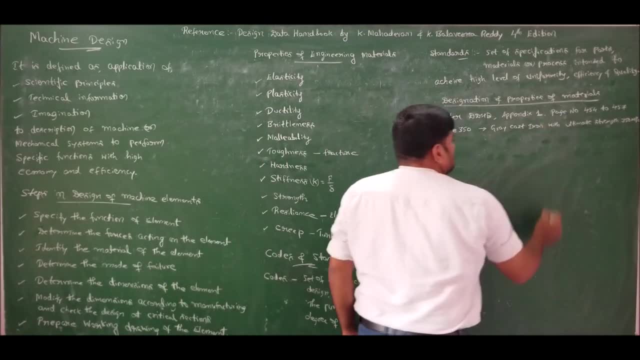 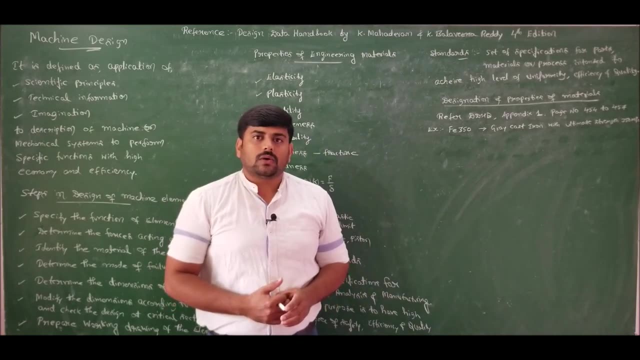 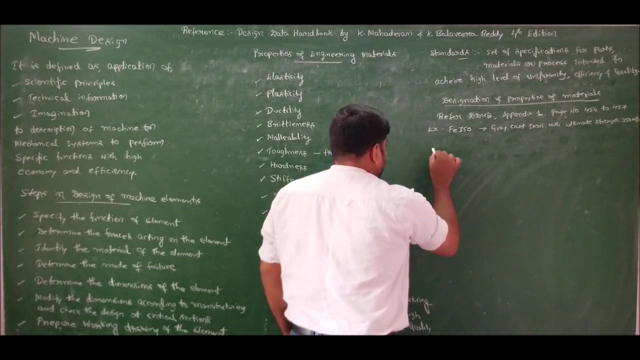 so this is about the introduction to this new course called machine design. as i said, i'll be dividing this entire machine design course into two parts, that is, design of machine elements 1 and design of machine elements 2. in design of machine elements 1, i'll be dividing it into 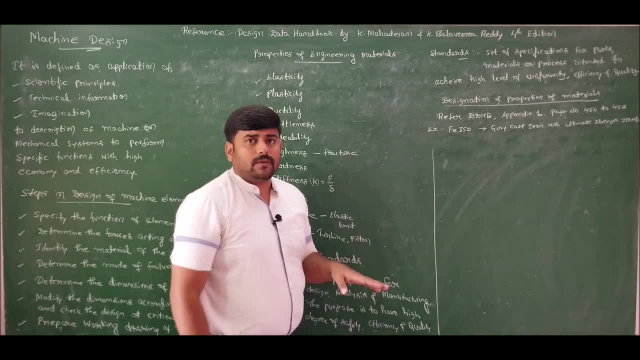 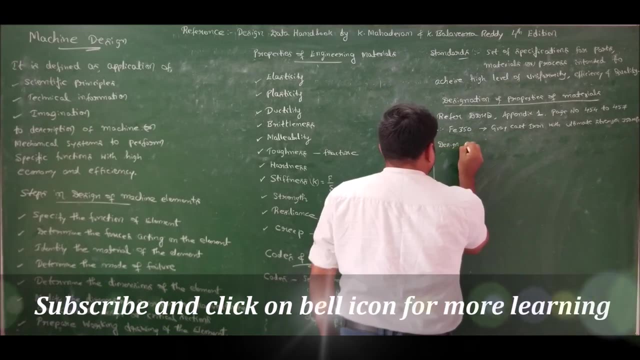 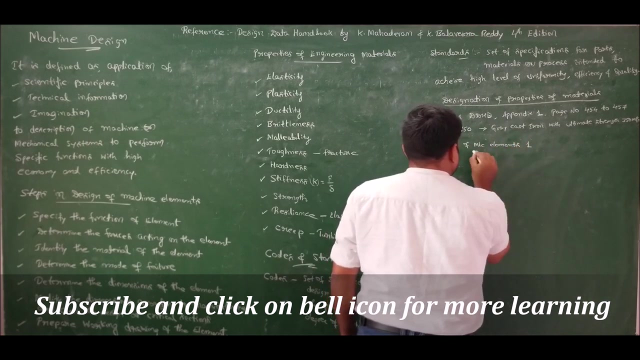 five modules and in design of machine elements 2 also. i'm taking up five modules in design of machine elements 1 in part 1. design of in design of machine elements, part 1. in first module i'll be addressing theories of failure, theories of failure and design. 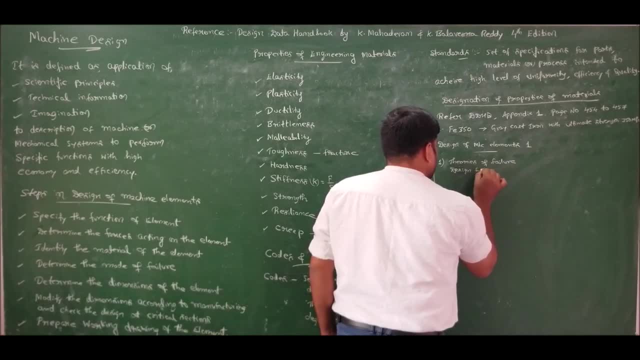 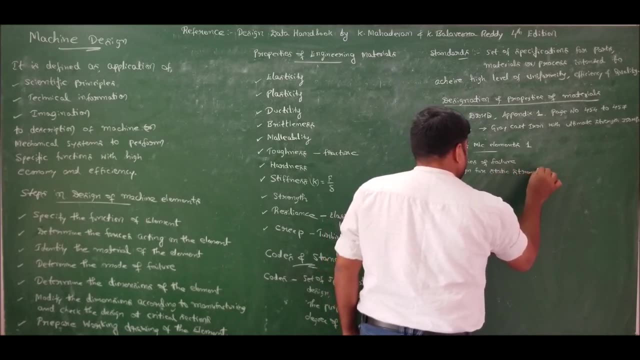 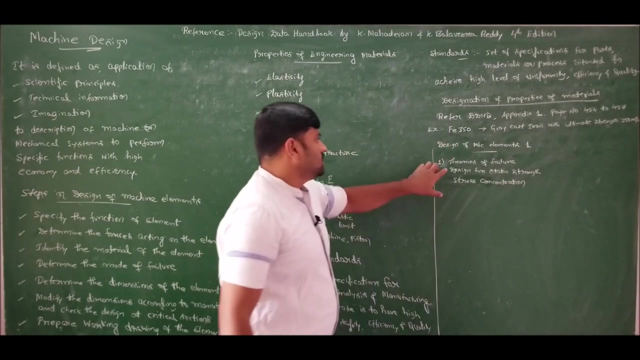 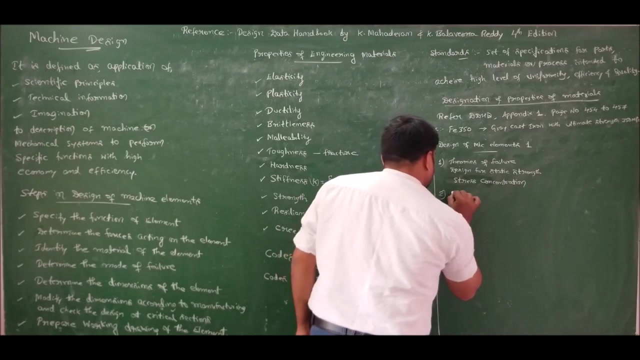 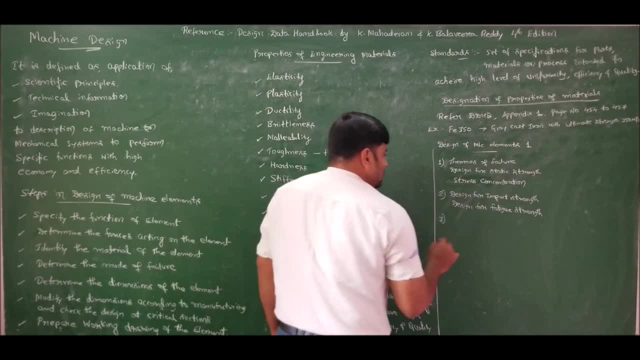 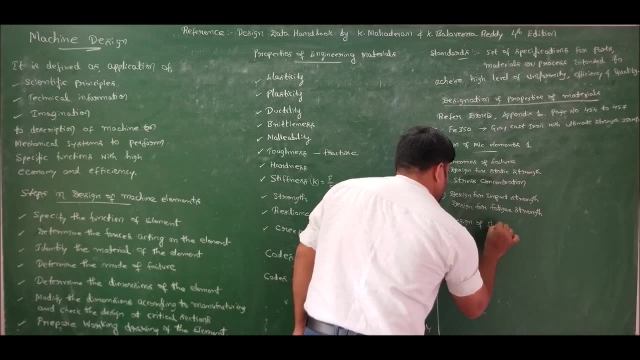 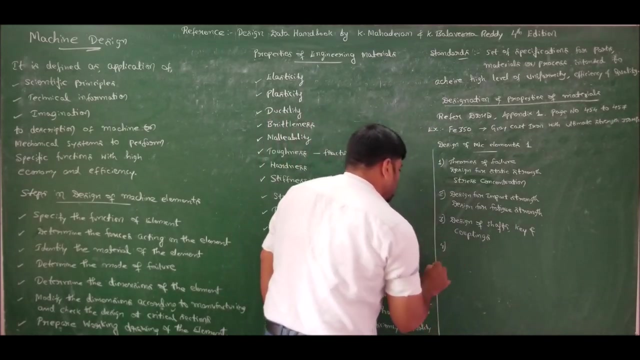 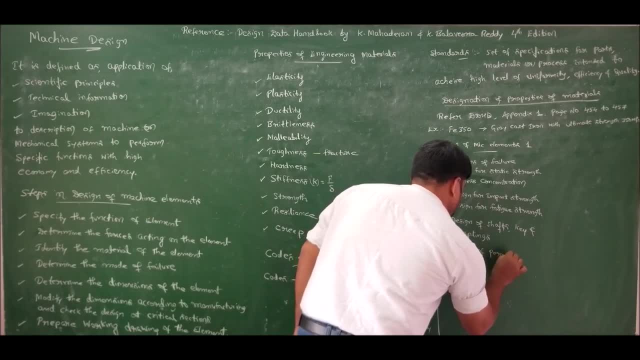 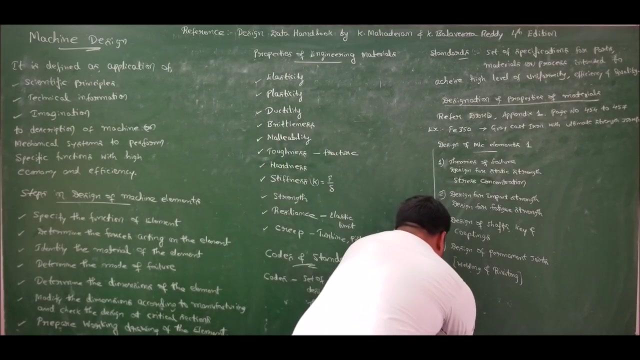 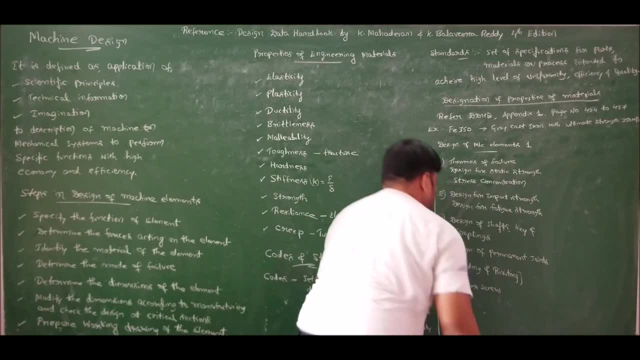 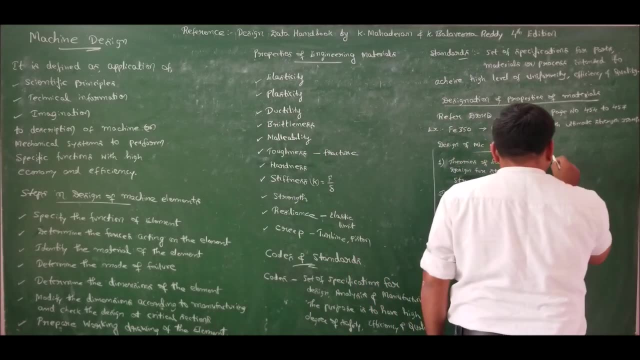 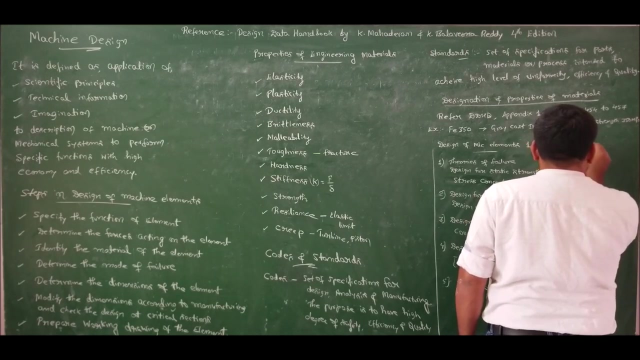 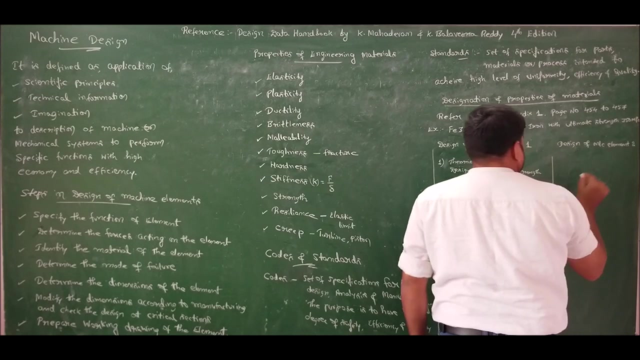 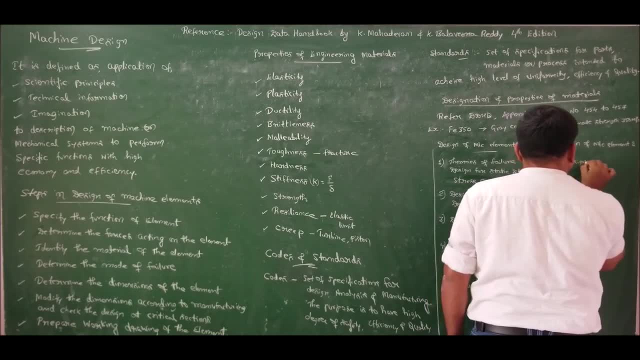 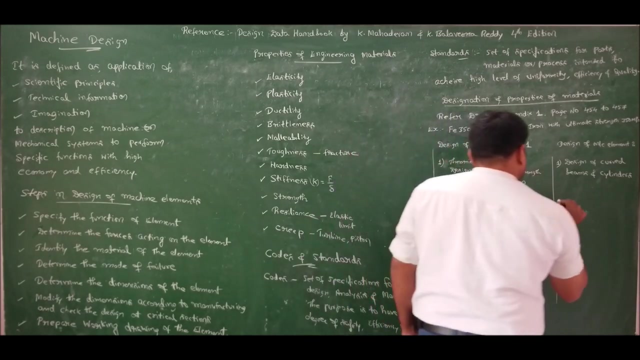 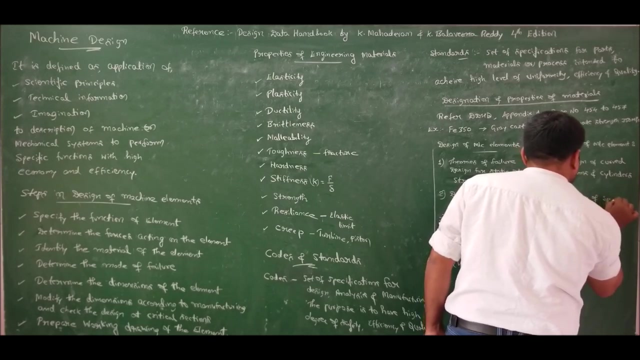 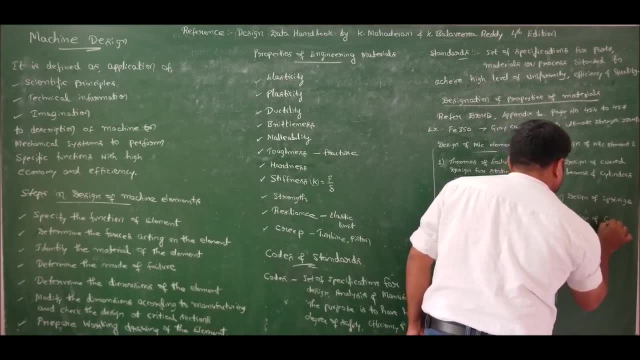 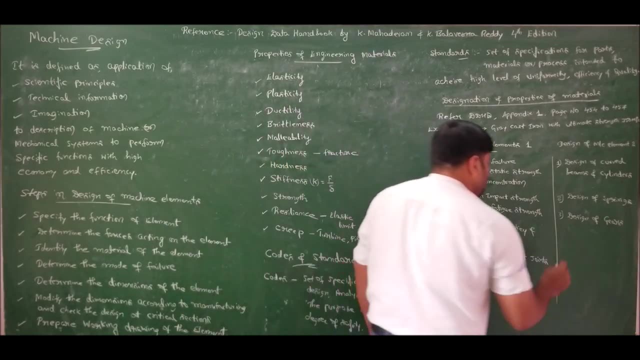 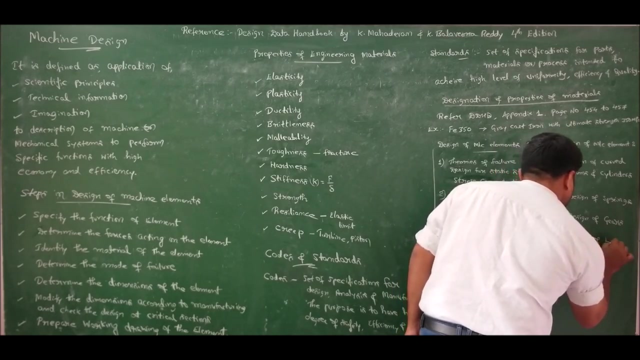 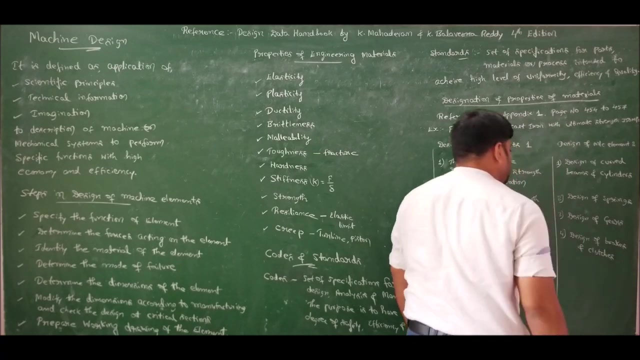 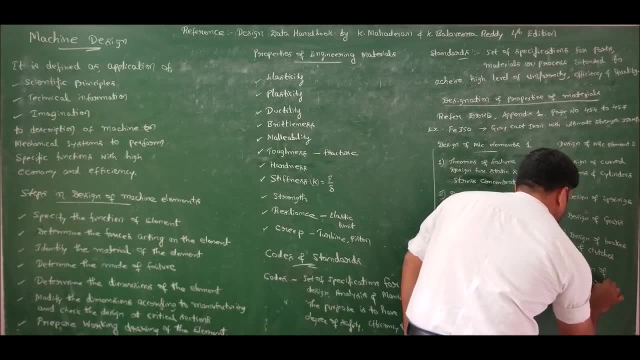 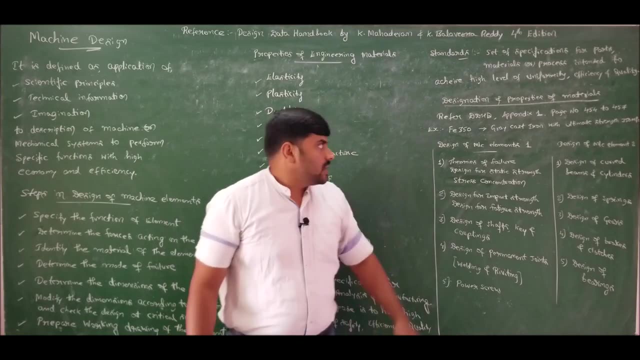 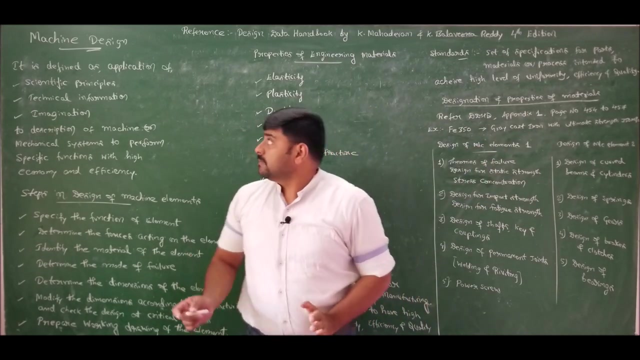 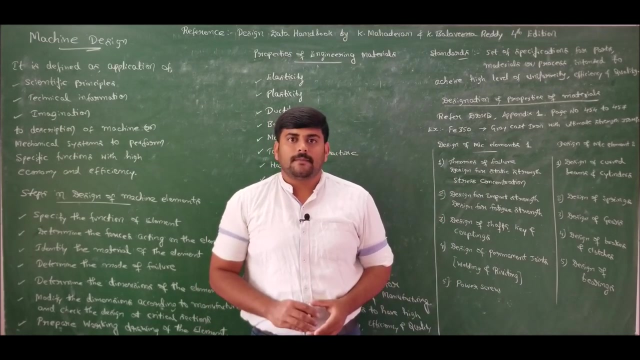